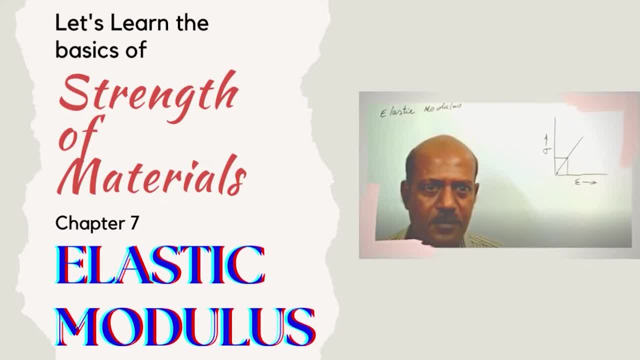 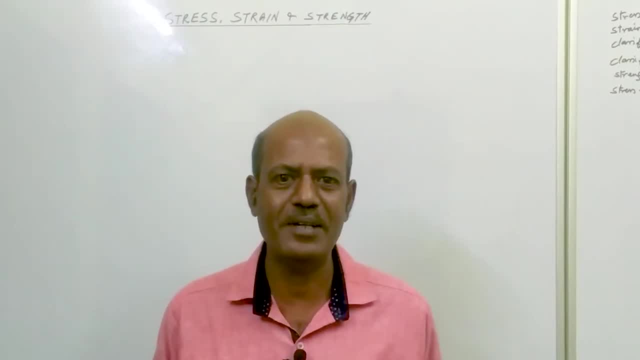 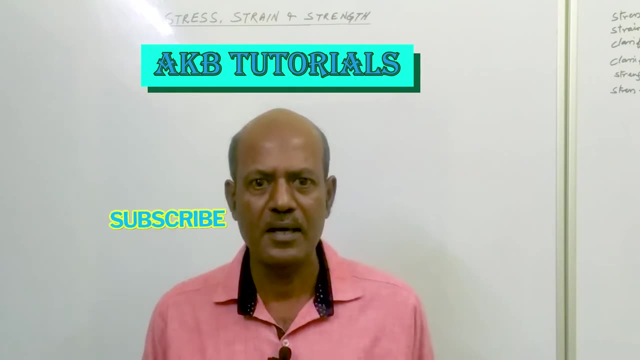 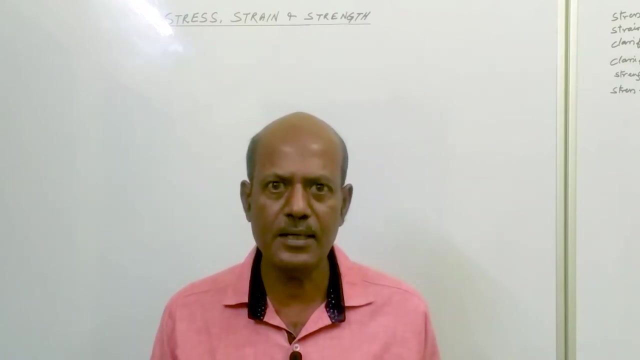 Hello everyone, this is Yashok, your personal guide and mentor. I welcome everyone to my YouTube channel, AKB Tutorials. Here we are going to discuss and cover some important concepts of mechanical engineering that are very useful and helpful for competitive exam and job interviews. So let us start today's session. So today we are going to learn one. 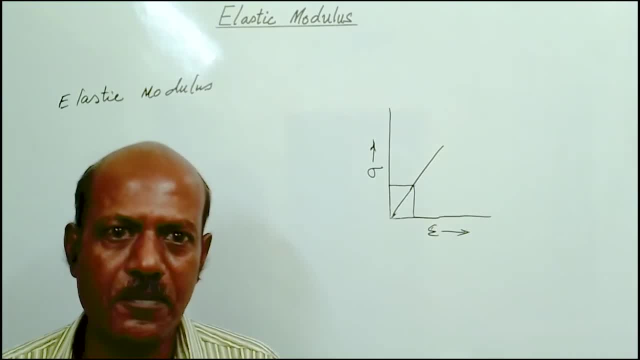 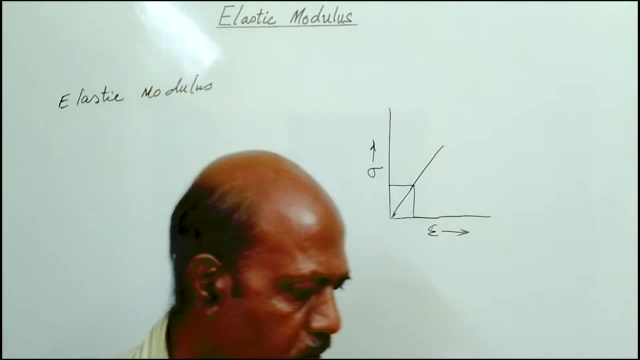 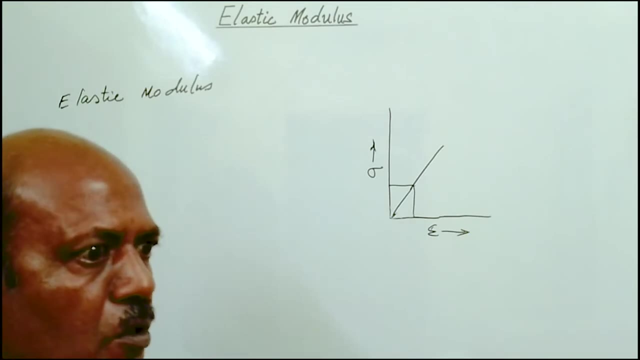 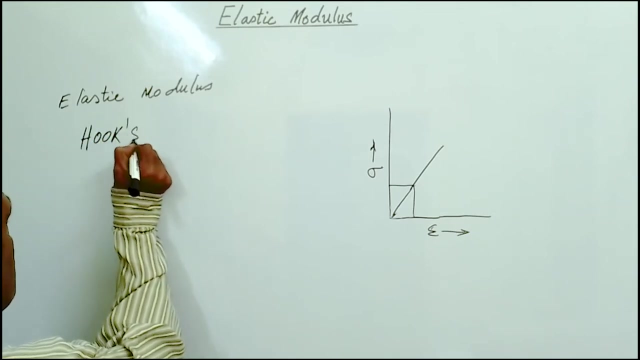 important topic of strength of material, That is, today's topic is elastic modulus. So today we are going to learn about elastic modulus. Now let us start with elastic modulus. So before going to elastic modulus, we will define what is called Hooke's law. So in basics we 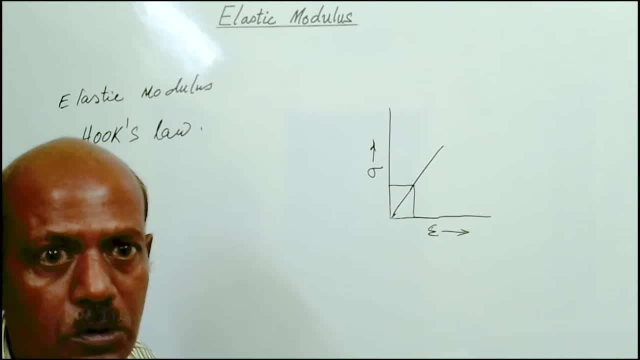 have studied what is Hooke's law. So Hooke's law is defined as: within elastic limit, the stress is directly proportional to strength. So what is Hooke's law? So Hooke's law is given by, within elastic limit, the process of intrinsic. 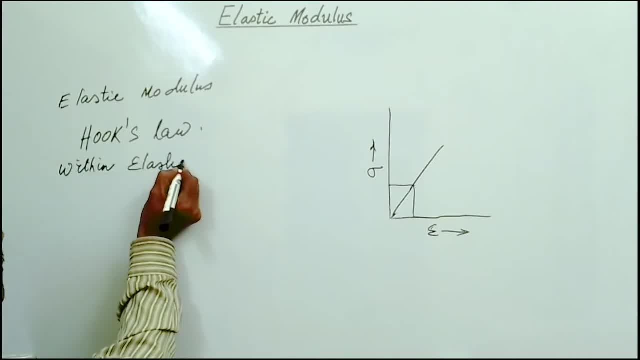 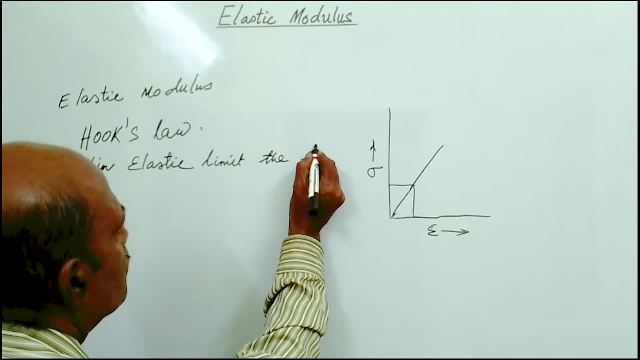 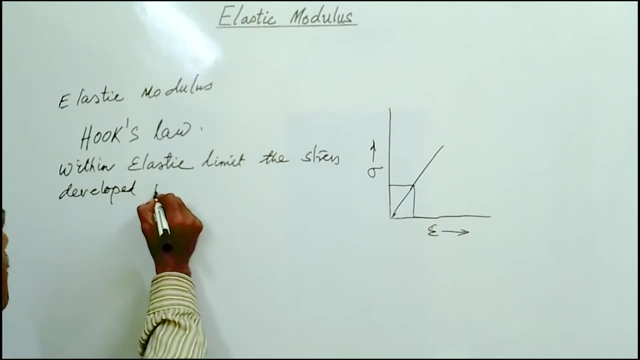 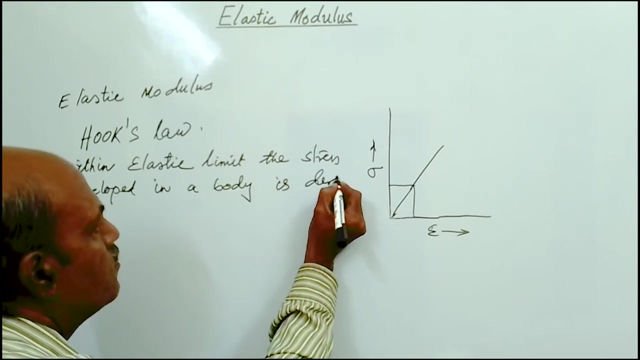 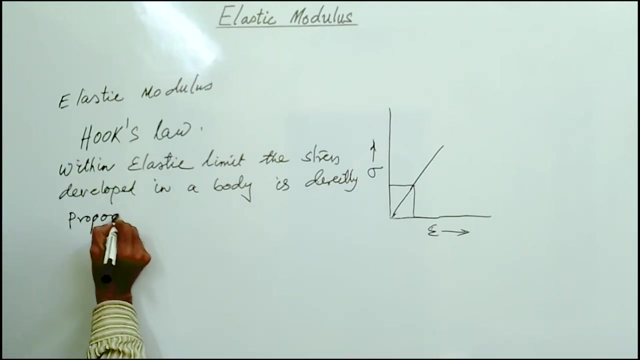 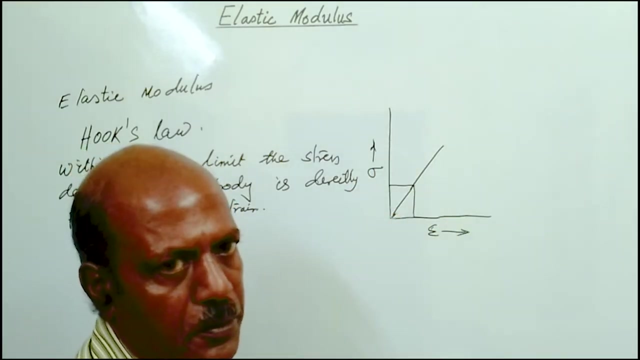 кого reasons. So this is given by: within elastic limit, the stress developed in a body is directly proportional to strength. However, within the sense that the So in a stress-train diagram, if we see within elastic limit, the curve is a straight line. 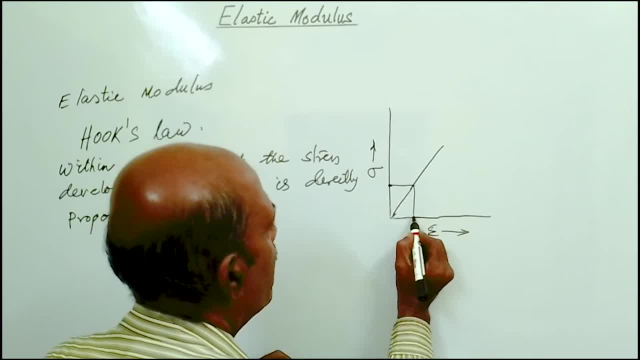 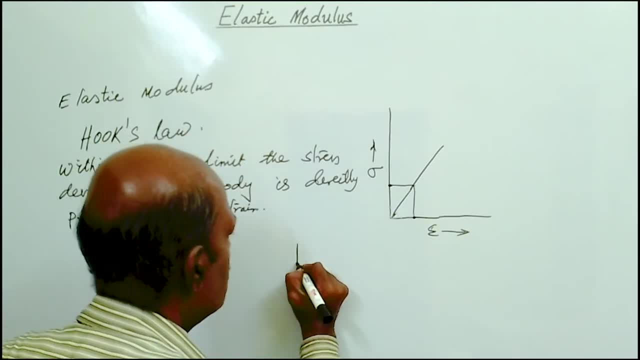 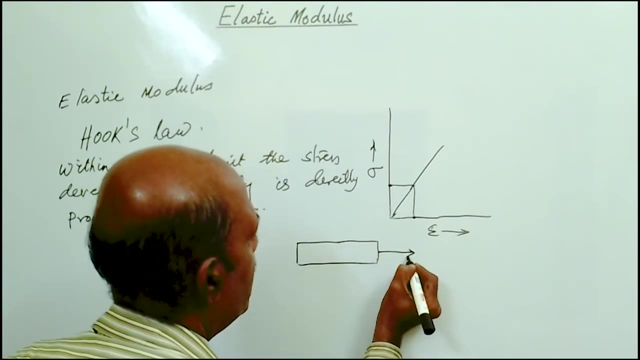 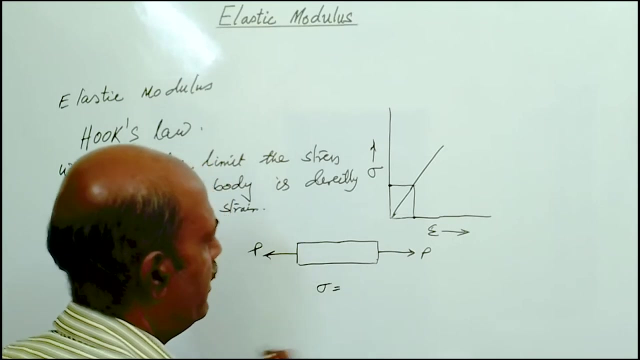 and this is the sigma developed in a body, and epsilon, that is strain developed in the body because of external load. So this is the body. The body is under external load, P. Here P is a direct load. Because of this P sigma developed in the body is given by P, by A, that is the strain developed in the body, by 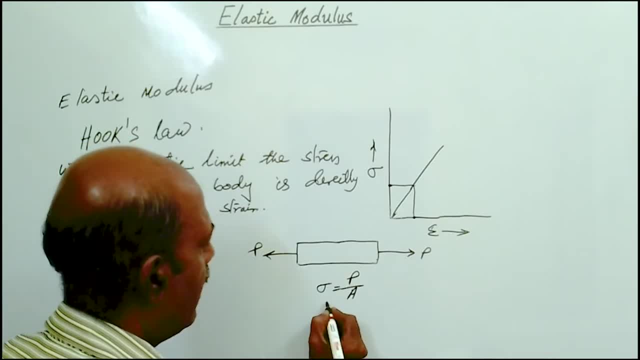 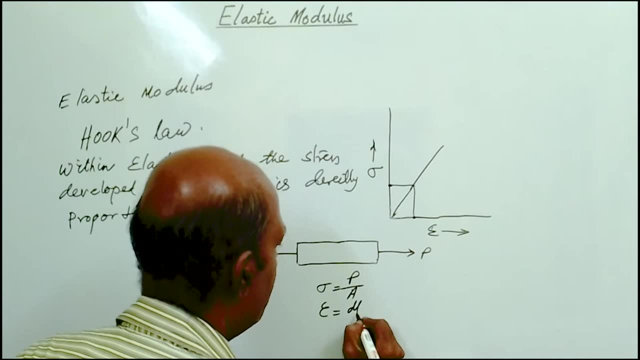 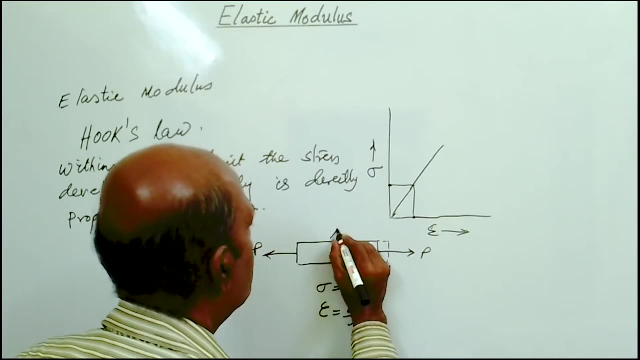 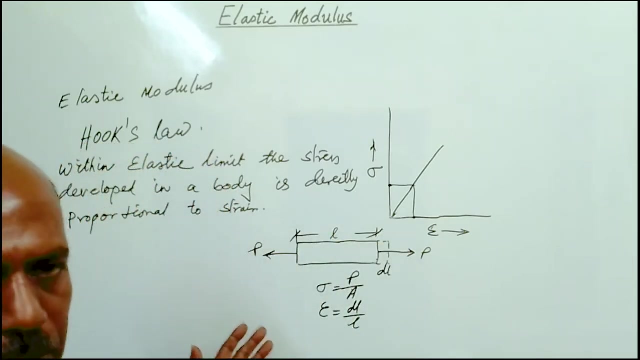 the original cross-sectional area and epsilon, that is, strain developed in the body, is given by. that is, dL, by L, where dL is the extension produced in the body over a length of L. So over a length of L, dL is the extension produced. 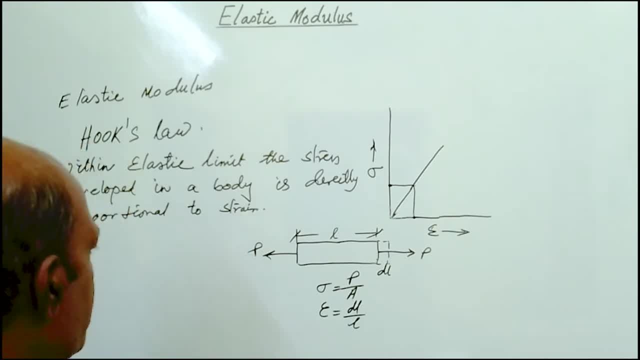 So dL by L is equal to the strain developed in the body. So as per the Hooke's law we can write: sigma is directly proportional to epsilon, or we can write: sigma is equal to some constant into epsilon. So here E is the elastic modulus. 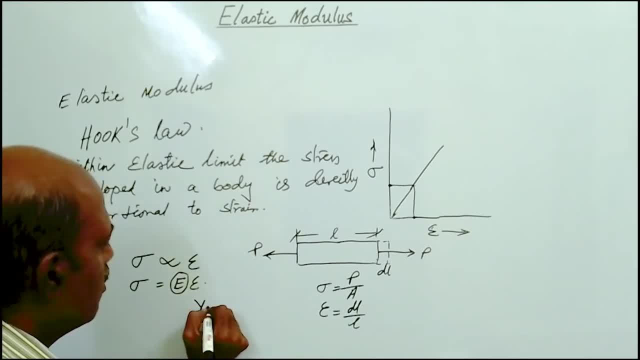 Now, what is E? E is known as Young's modulus of elasticity, Young's modulus. So what is Young's modulus of elasticity? E is given by sigma, by epsilon, where sigma is known as direct stress, because the stress produced because of the direct load. 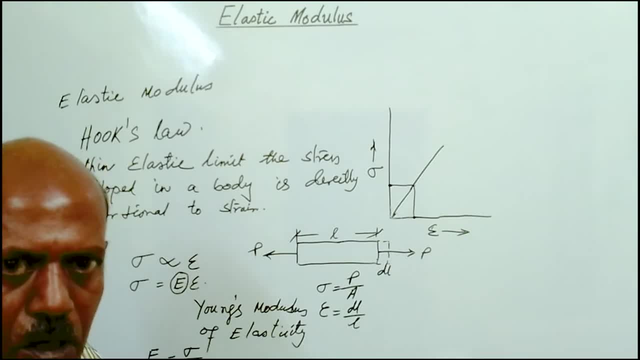 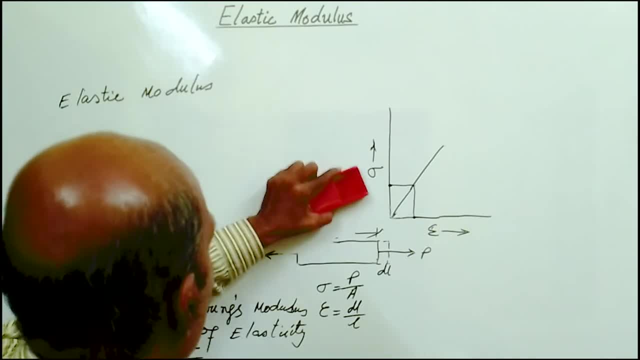 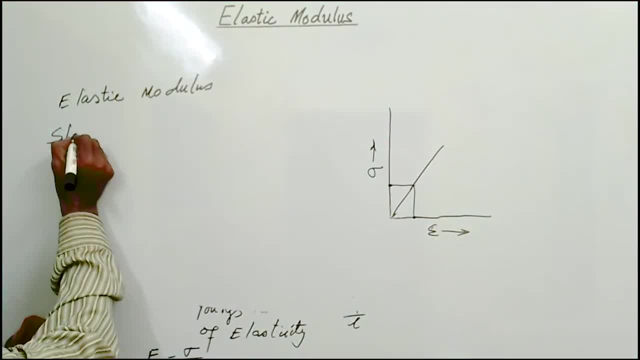 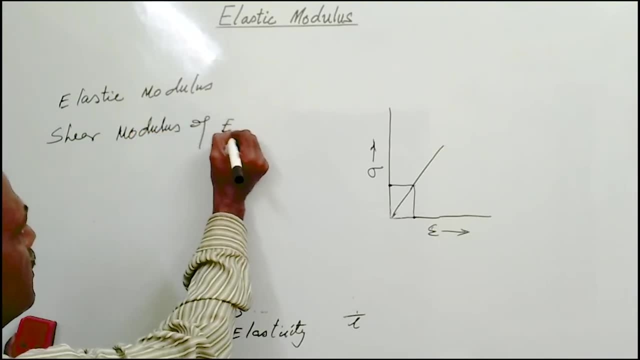 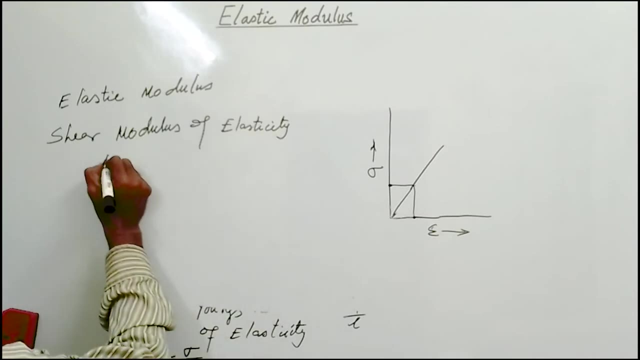 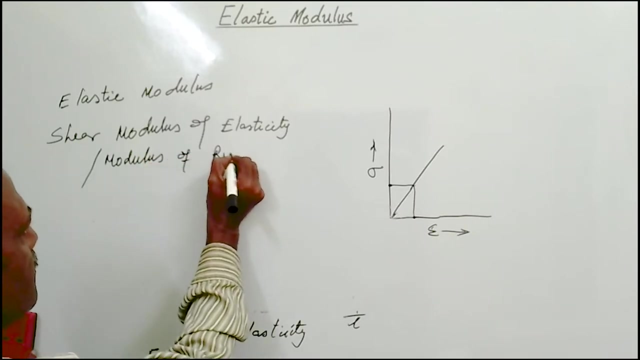 load. So E is given by sigma by epsilon, where sigma is known as direct stress because of the direct load, So E is given by sigma by epsilon, where sigma is known as direct stress because of the direct load. are modulus of elasticity, or is also known as modulus of rigidity or modulus of rigidity. 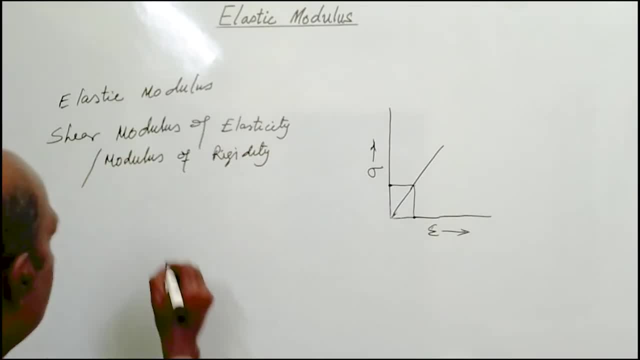 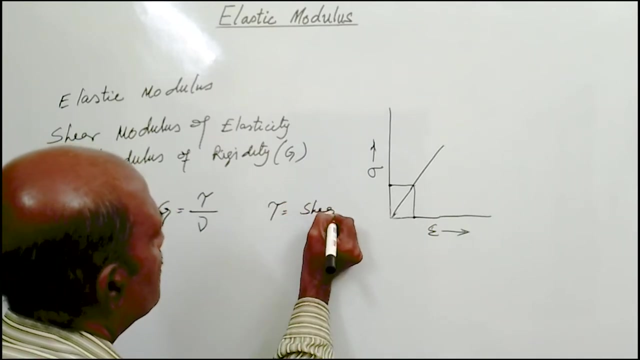 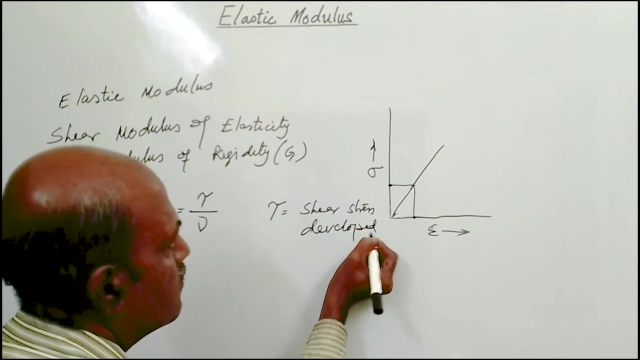 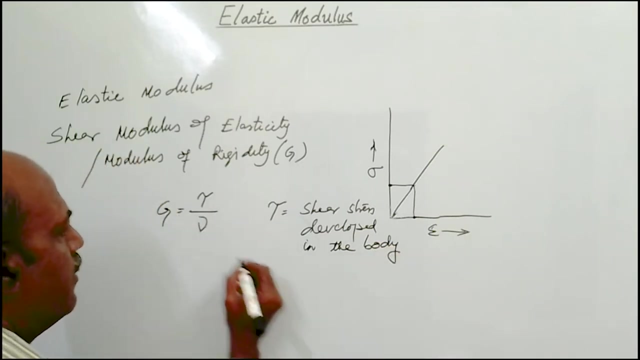 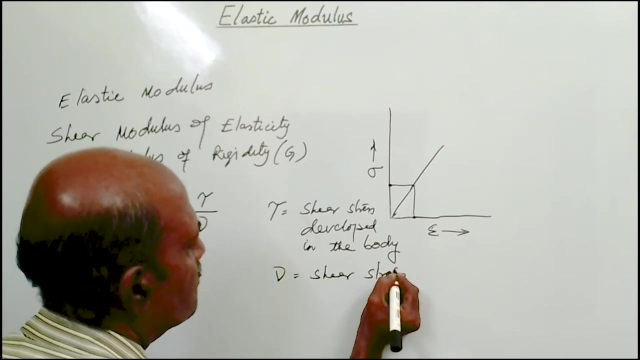 So this is defined as: as denoted by g. modulus of rigidity is denoted by g, where g is equal to tau, by, say, gamma, where tau is the tau is the shear stress developed in the body, shear stress developed in the body, Body because of shear load, and gamma is equal to shear strain. 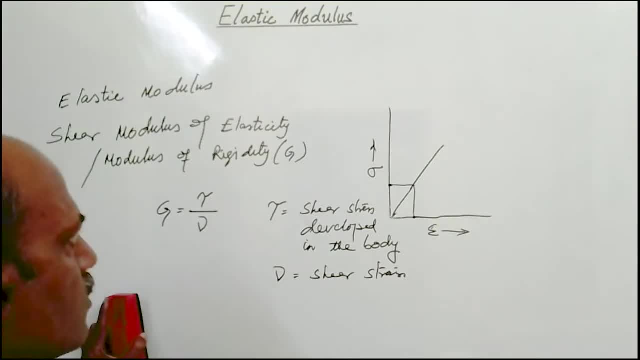 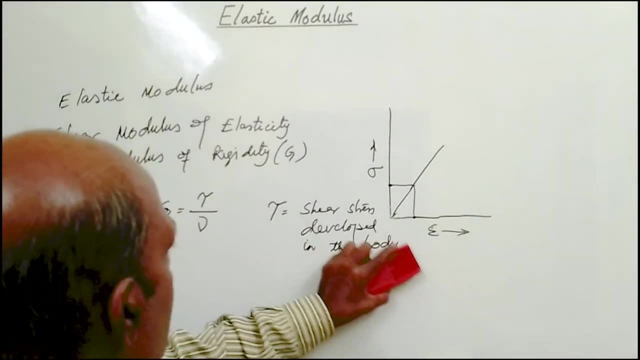 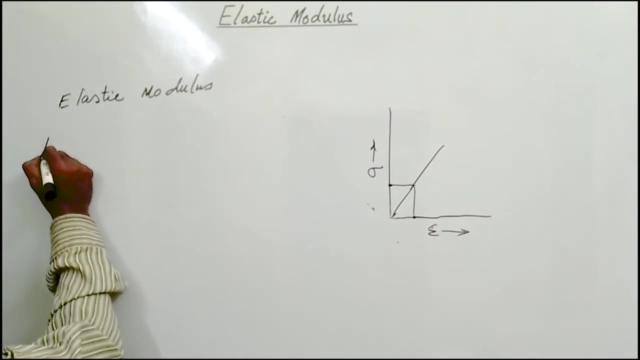 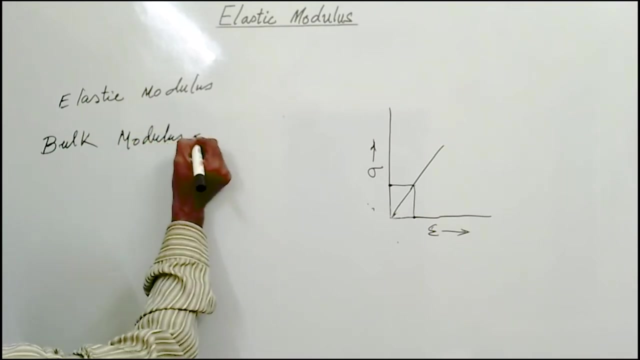 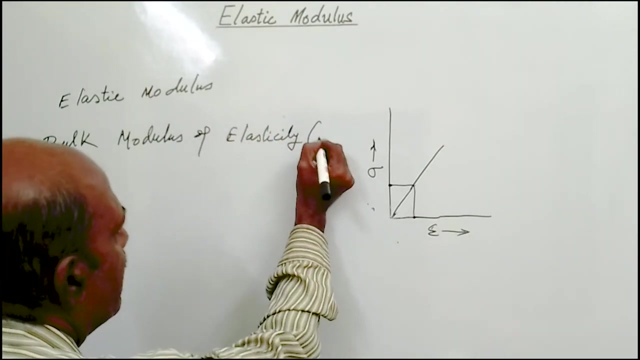 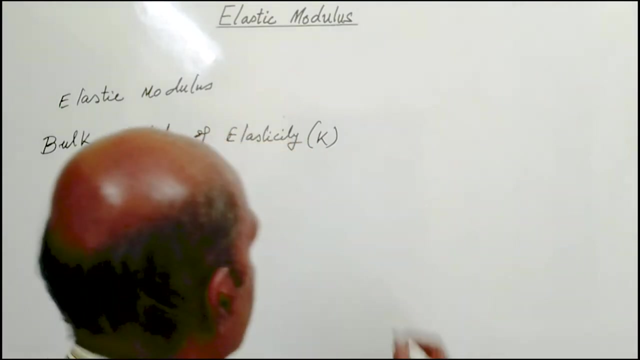 So the ratio of shear stress to shear strain is called modulus of rigidity or shear modulus of elasticity. Now the next modulus, that is Bulk modulus of elasticity. bulk modulus of elasticity, and it is denoted by k. Bulk modulus of elasticity is denoted by k. 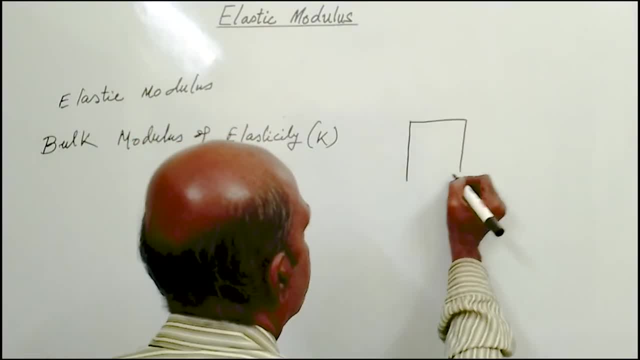 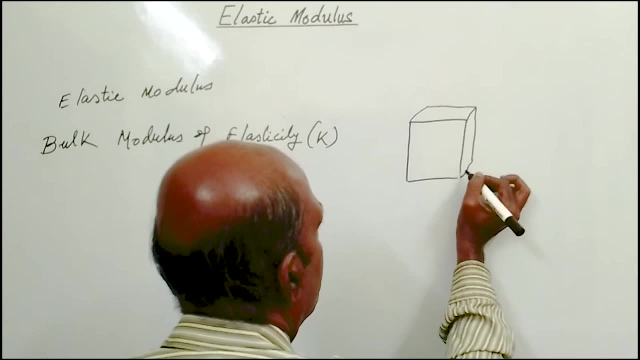 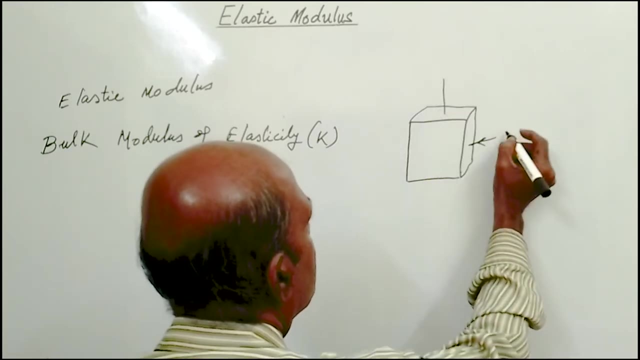 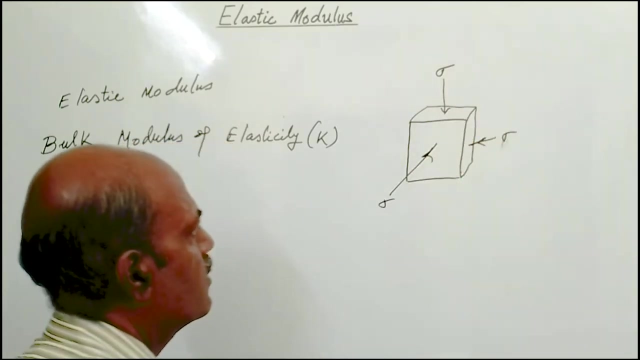 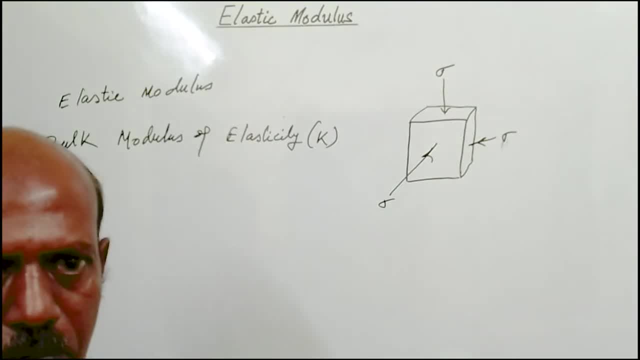 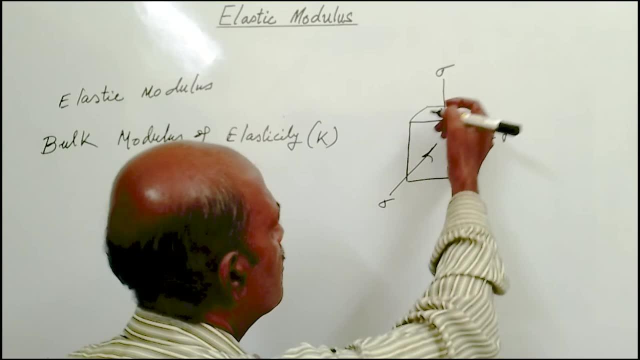 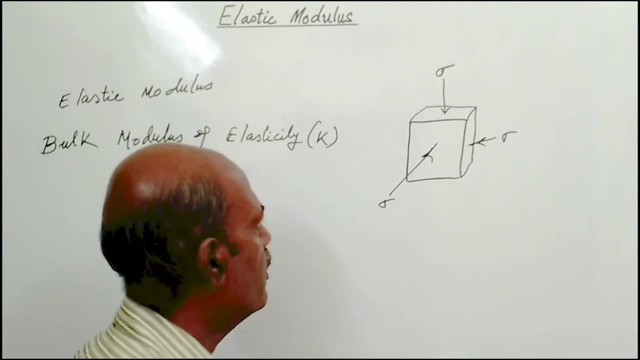 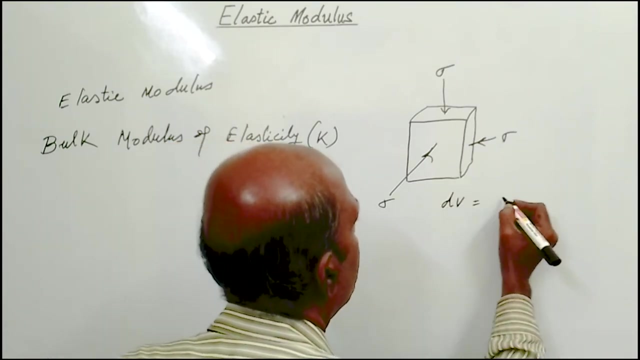 So uniform stress is acting over the body from all the directions And because of this Stress, So some Means, Because of this compressive load, some strain is developed in the body, Means the volume of the body will change. let change in volume is given by dv. 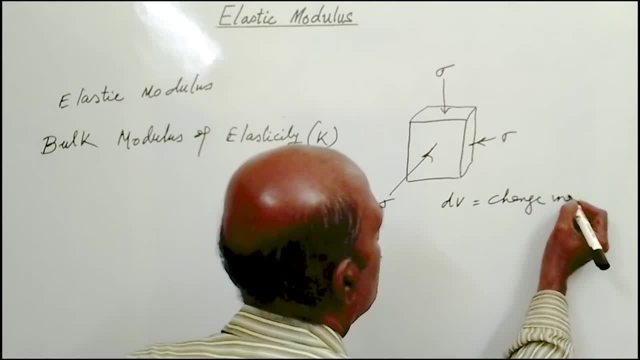 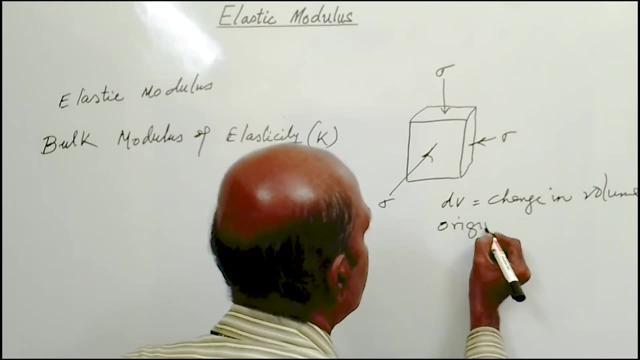 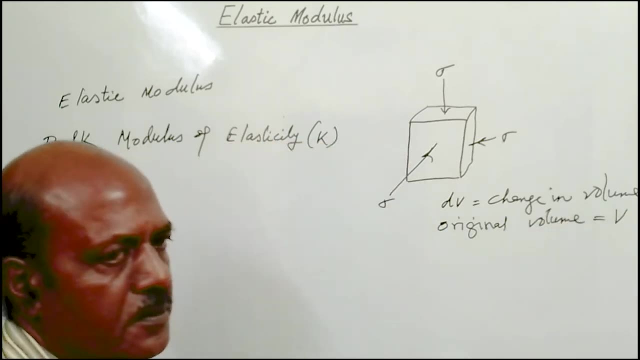 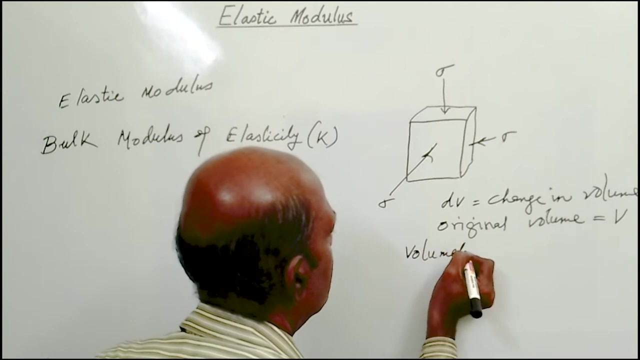 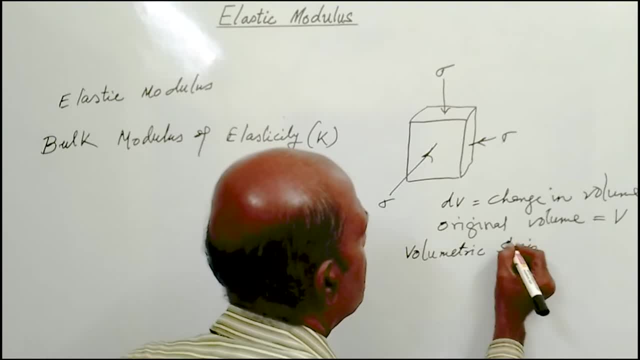 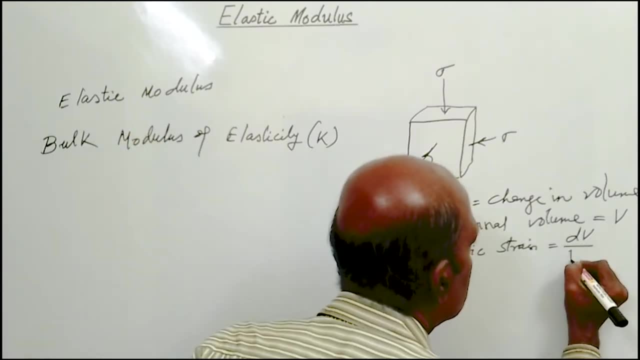 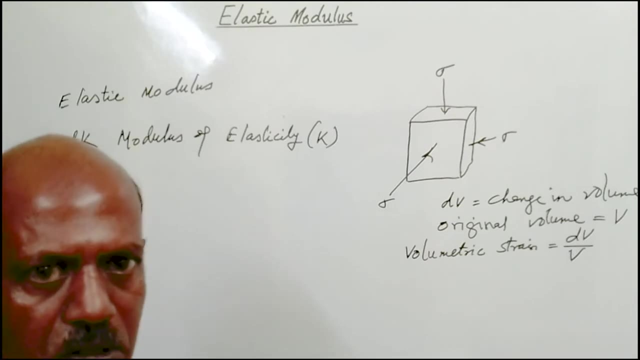 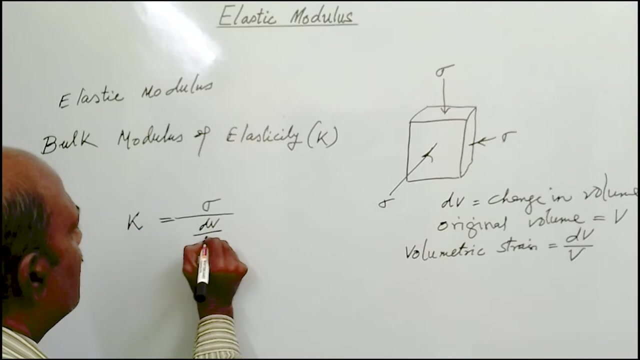 Bulk Bulk. Bulk In the normal Bulk because of the load is compressing load acting over the body. so volume at extreme is given by dv, by v. now bulk modulus of different elasticity is defined as bulk modulus of elasticity. k is equal to uniform stress intensity. say sigma by dv, by v. 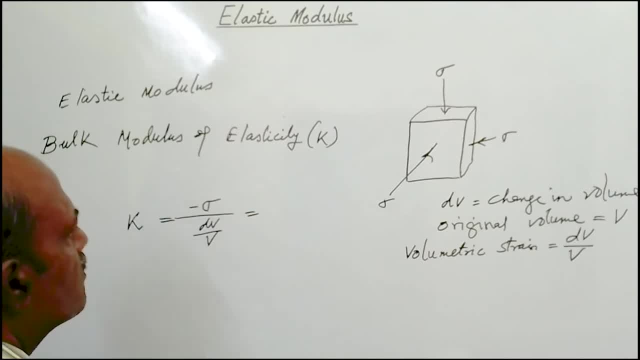 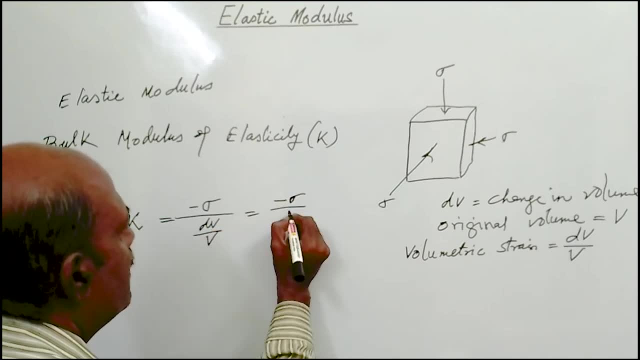 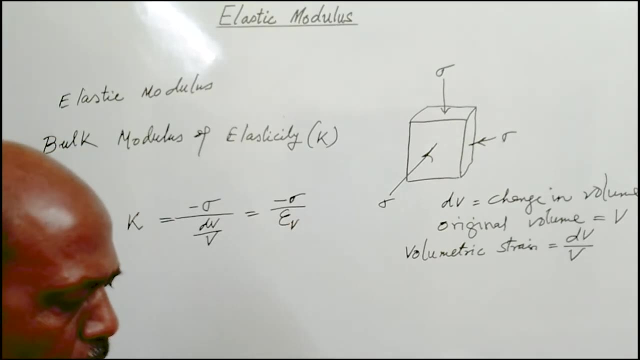 so it is given negative sign because stress is negative. so minus sigma divided by dv, by v, is that volumetric strength. so it is denoted by epsilon v. so we have seen the three elastic constant. what is e, g and k? that is young's modulus of elasticity. 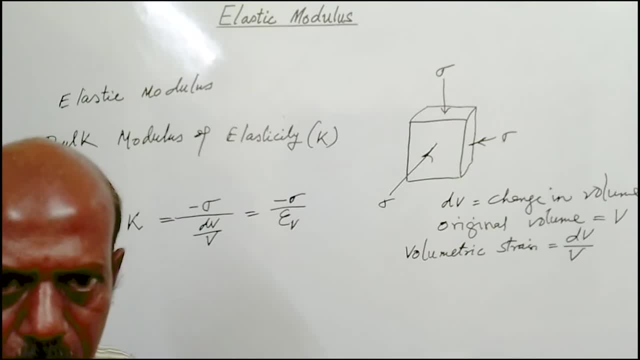 over in stress and strain are direct stress and strain acting over the body. so that will produce: that is young's modulus of elasticity. then next point: shear stress injecting over the body. that is bulk modulus of elasticity. sorry, shear modulus of elasticity. g is given by tau y gamma shear stress to shear strain and and k is the bulk modulus of elasticity. 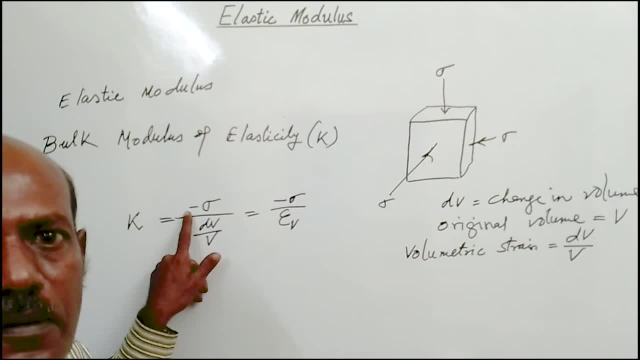 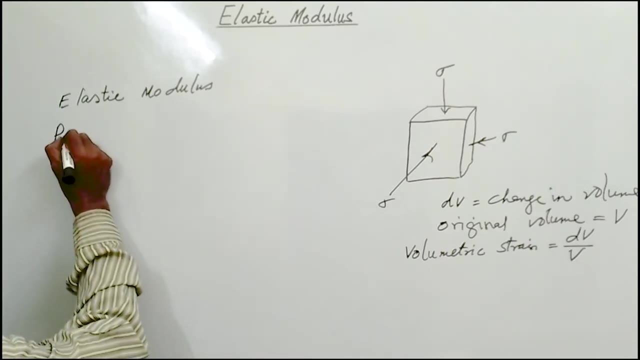 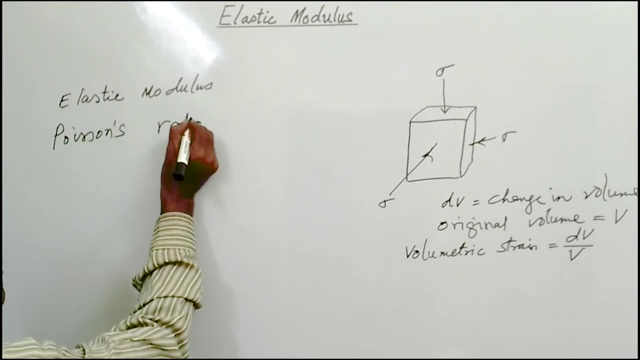 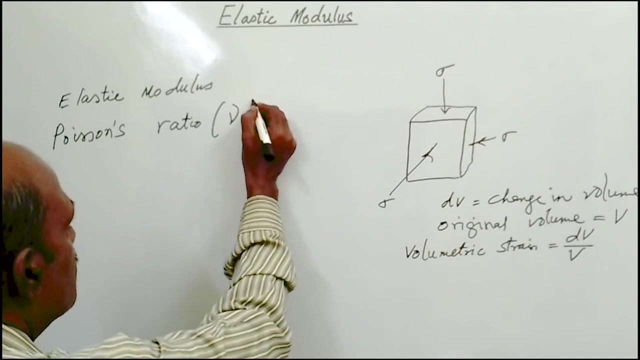 that is given by the ratio of uniform stress intensity to to the volumetric strain. now we will see that another elastic constant that is called the poisson's ratio, poisson's ratio. so poisson's ratio is denoted by mu and mu is given by that is lateral strain. 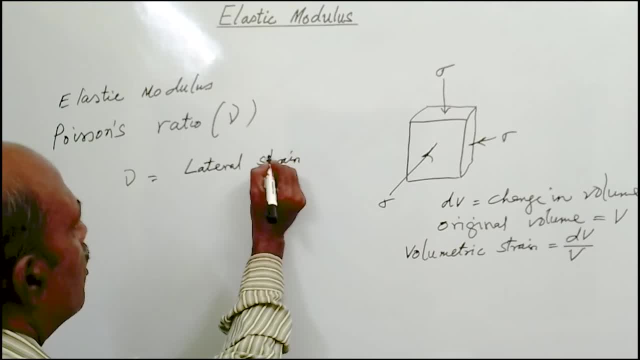 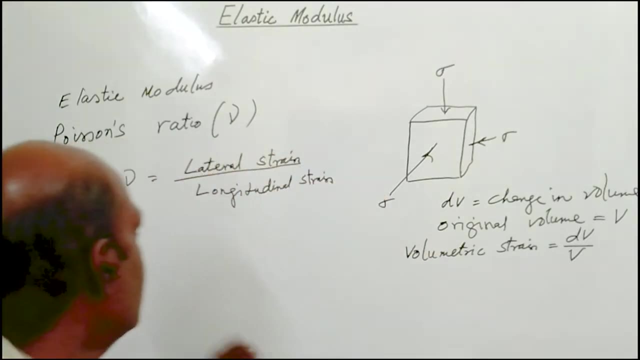 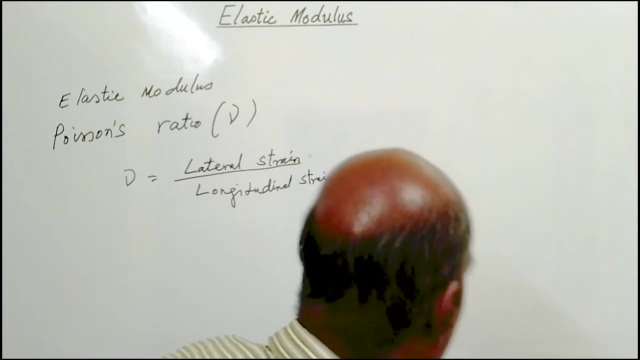 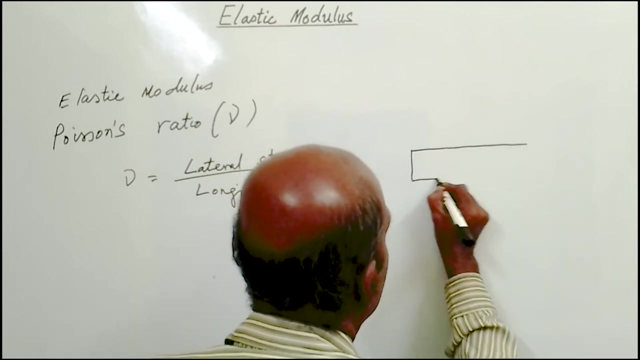 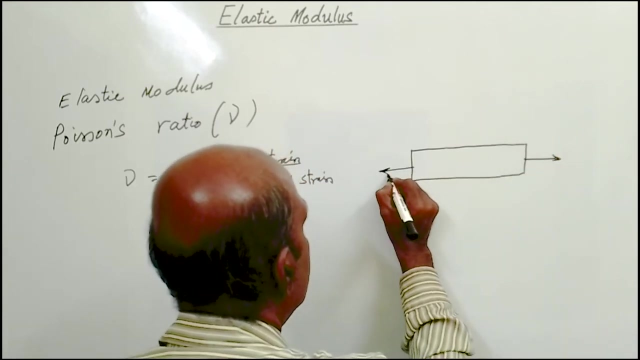 lateral strain to to longitudinal strain. so, similar to a lateral strain, an unravels from diagonal over to non-vegetarian structure. so we should learn what is lateral strain and longitudinal strength. then it will be clear. that is say a body, body is of three-dimensional body, this is the three-dimensional body. 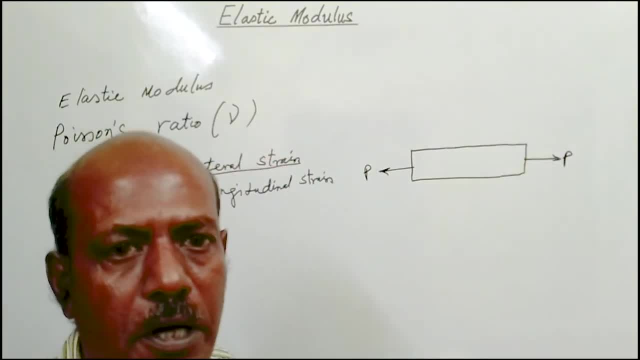 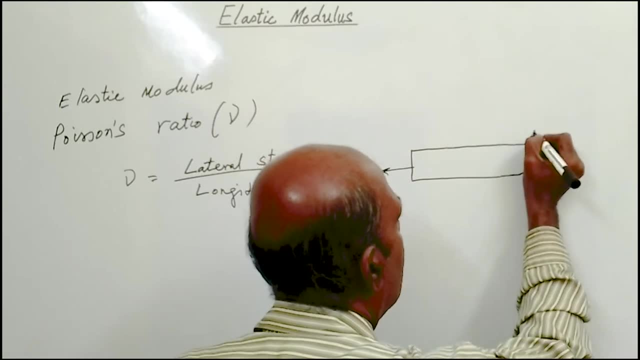 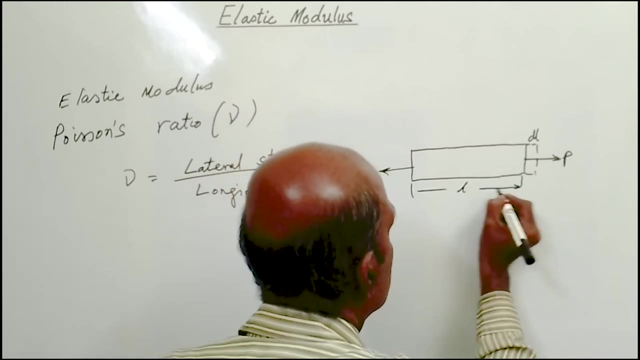 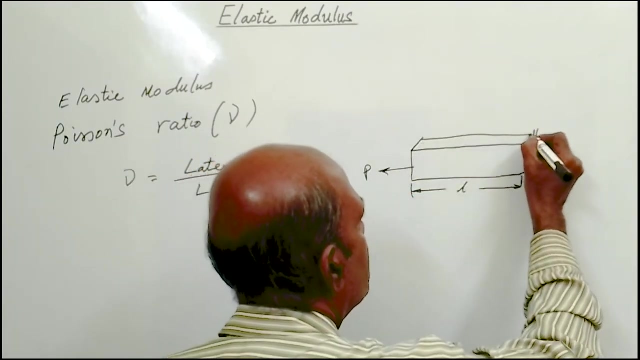 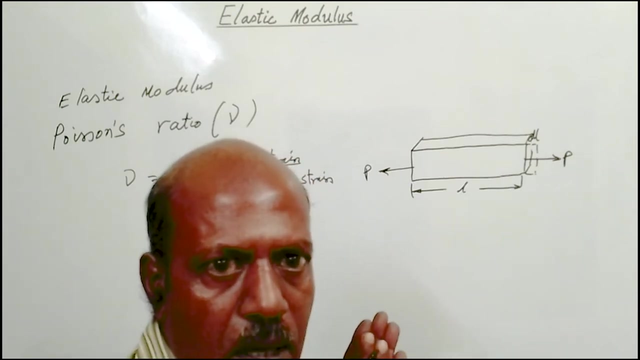 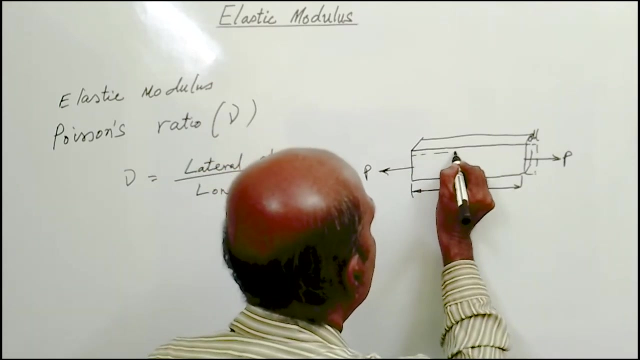 Because of this direct load acting over the body, the deformation in the direction of load will take place. say, DL is the deformation over a length of L. So let's see the three dimensions of the body. Now, once the body elongates along the direction of load, so other directions, that is perpendicular. 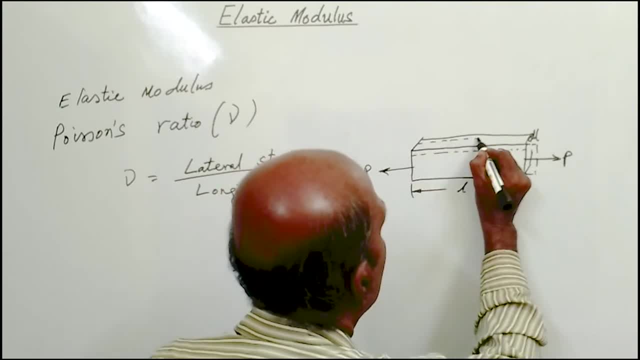 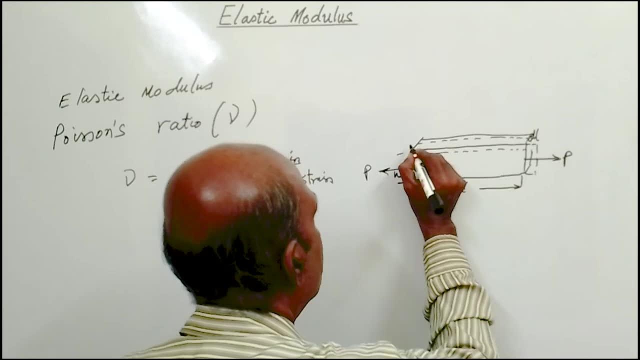 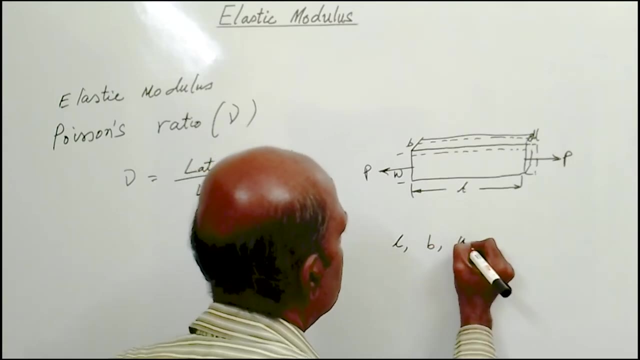 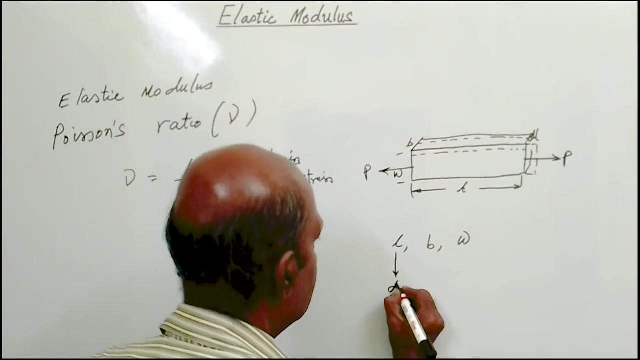 to the load, it will decrease. Say the dimension L and this dimension is W and this direction length is B. So L is the length, B is the width and W is the thickness of the body. L is the width. Now, in along direction L, DL is the increase in length because of direct load. P is acting. 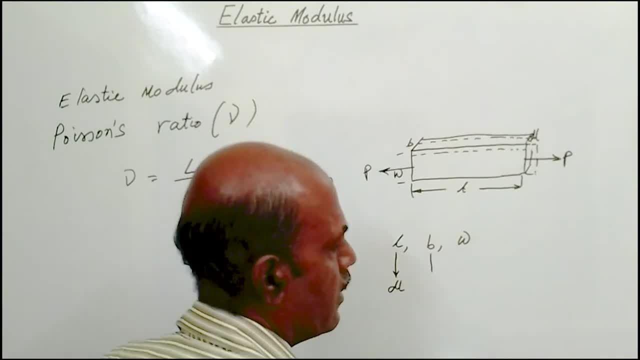 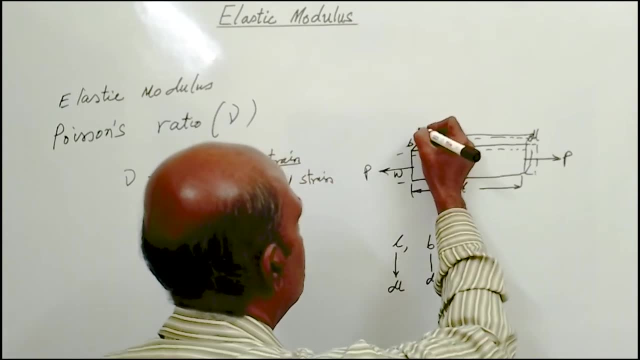 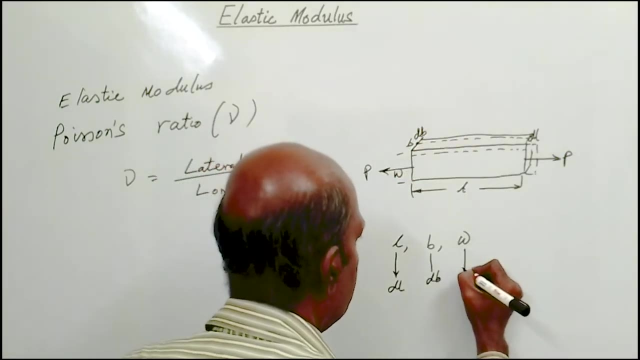 along length L and along direction B, so there will be some change. say DB is the change, So DB is the change, means it will reduce in size. Similarly, along direction L, DL is the increase in length And along direction W, change is DW. 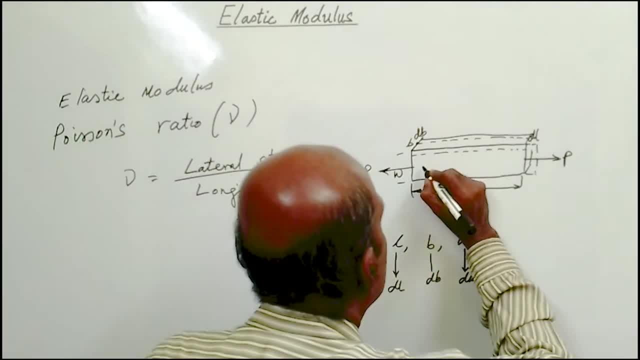 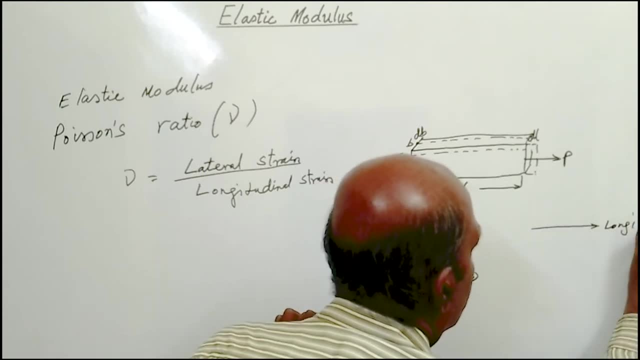 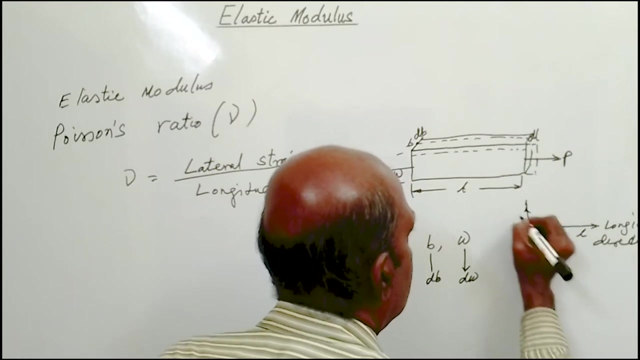 So this direction, the direction along the direction of the load, is called longitudinal direction. longitudinal direction So there are other two directions, that is along the direction of W. so this is the direction L, this is the direction W and this is the direction B. 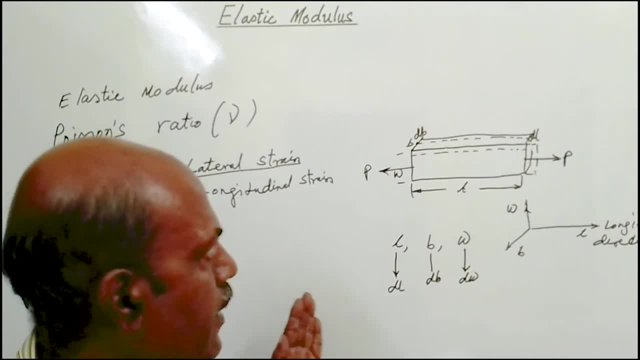 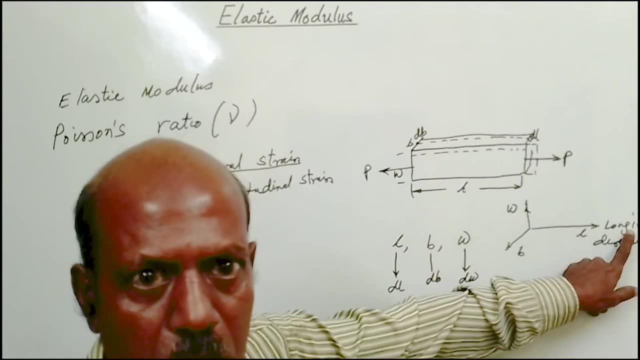 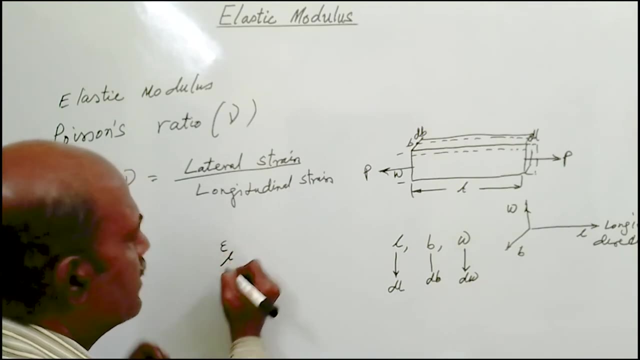 So whenever a load P is acting along length L, so L will increase and it will produce longitudinal strain in this direction and is given by, say, epsilon: L is the longitudinal strain produced in the body. It is given by DL, by L And in other two directions perpendicular to L, direction, that is, B, and 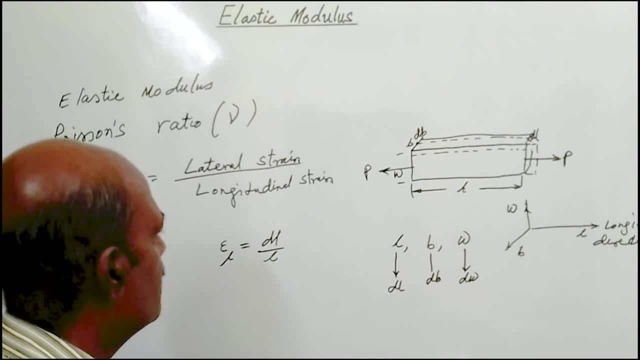 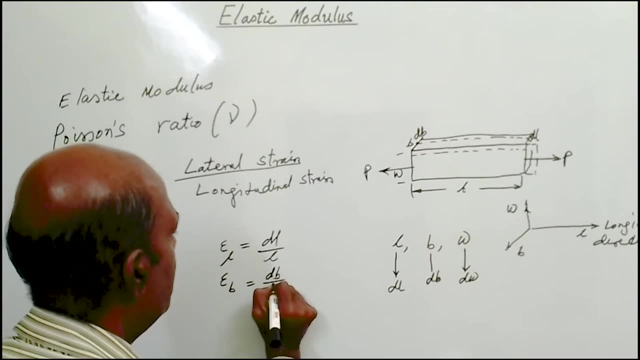 W direction. the strain will be a compressive strain and it is given by epsilon B is equal to DB by B and epsilon W, that is along direction W strain produced- is given by DW by W. So that is along the direction W the strain will be a compressive strain and it is given 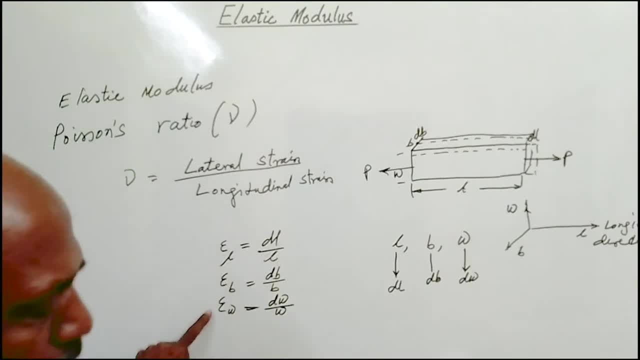 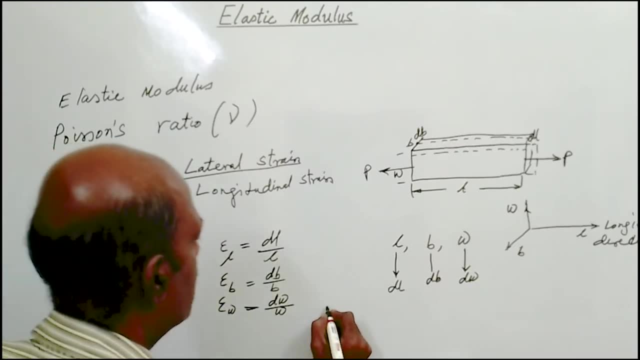 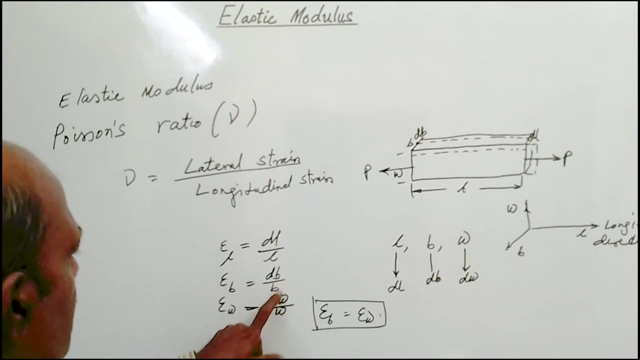 by DL, by L, And this EB and EW are called lateral strain and EL is called longitudinal strain. So these two, that is epsilon B and epsilon W, are equal. So within elastic limit, the ratio of lateral strain either epsilon B or epsilon W divided. 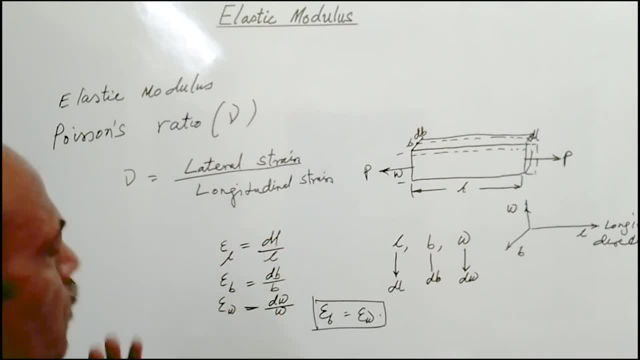 by the longitudinal strain, that is, epsilon L, is known asDL by DL, by DL by DL, as poisson's ratio, and is given, denoted by nu, that is, that is epsilon b or or epsilon w divided by epsilon l is called the poisson's ratio. now we'll see the relation between the elastic 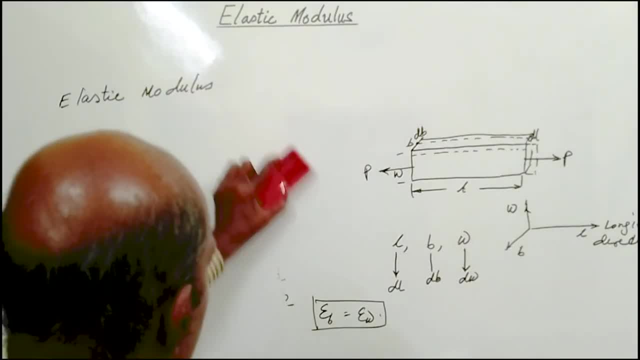 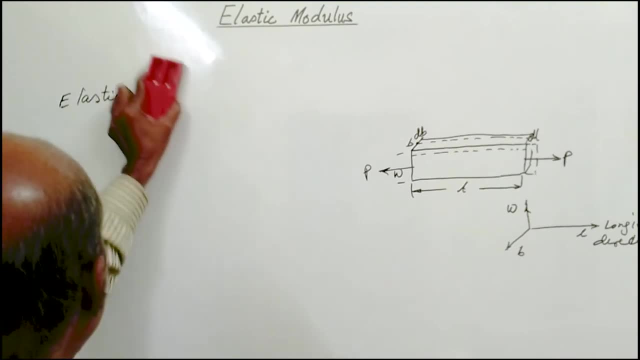 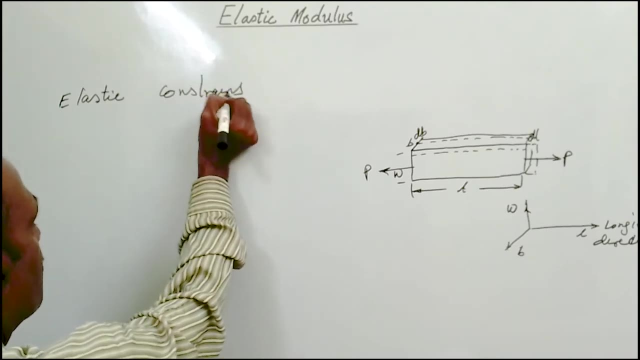 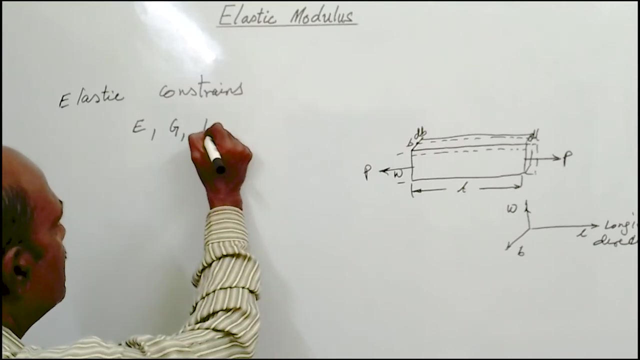 constants. so there are four elastic constants in strength of material. what we are saying so that we write elastic constant or elastic modulus, elastic constant or elastic modulus. there are four elastic constant, that is e, m, modulus of elasticity. second one is g, modulus of rigidity. then third one is k, that is valve modulus of elasticity. and fourth one is: 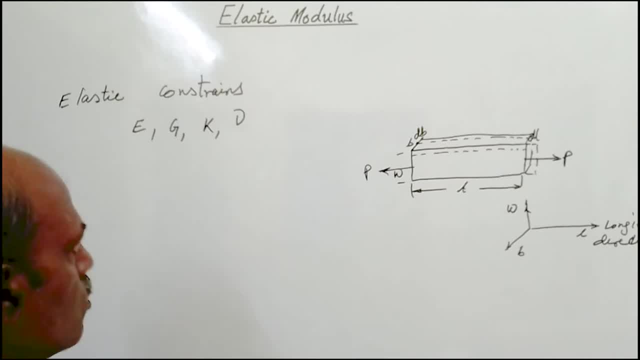 nu, that is poisson's ratio. so so if we know any two of the elastic constant, any two elastic constant, then for a isotropic material the property can be defined properly or completely. so properties of an isotropic body can be defined completely if we know any two of these properties. 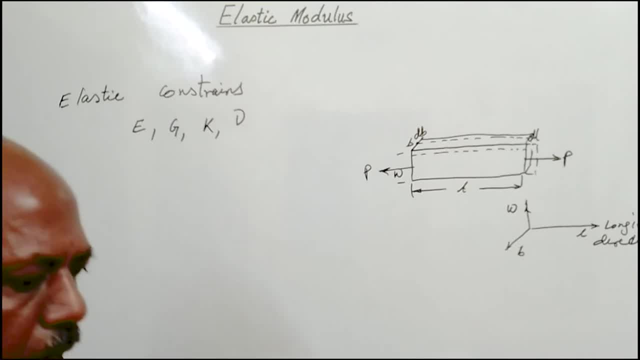 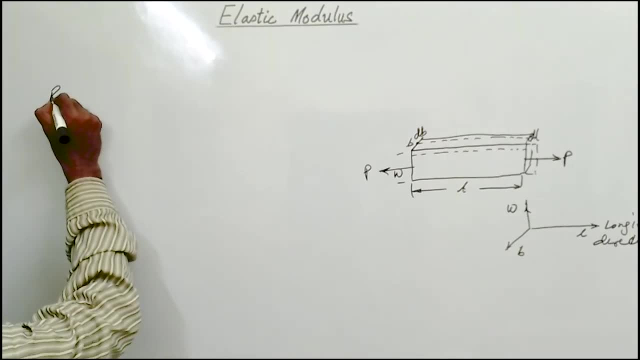 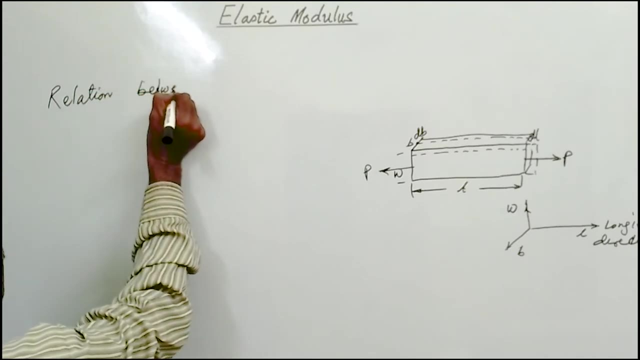 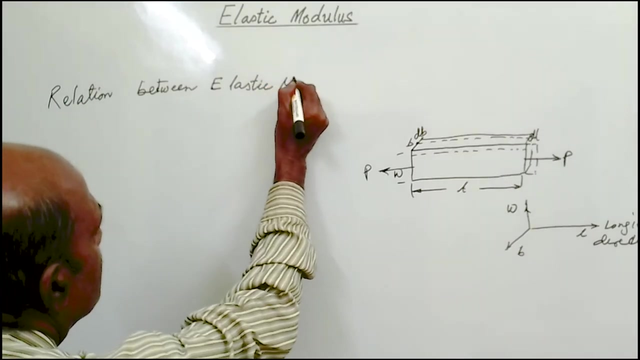 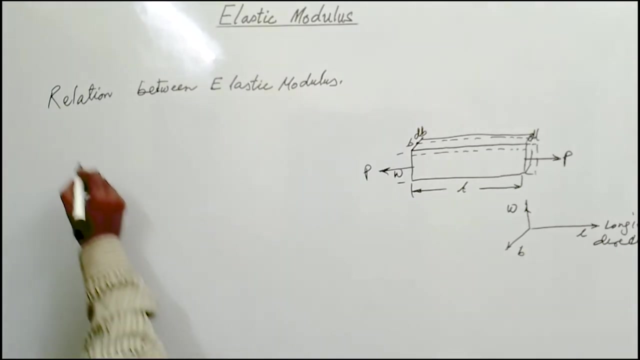 so now we'll see the relation between the elastic modulus or elastic constants, that is relation between. So the first relation, that is relation between E and G, relation between E and G, that is Young's modulus of elasticity and modulus of rigidity. So there is a small proof, given in every book. 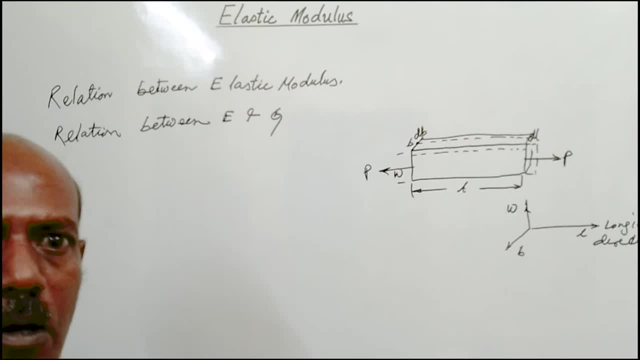 So you can directly write this and you have to remember this for solving the problem as well as for any competitive exam. these questions may come directly. So E is equal to 2G into 1 plus mu. So this is the relation between the. 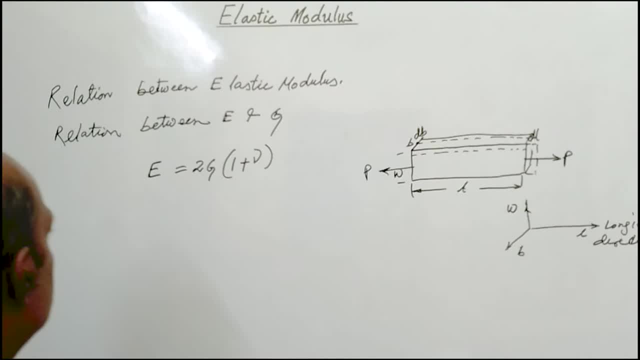 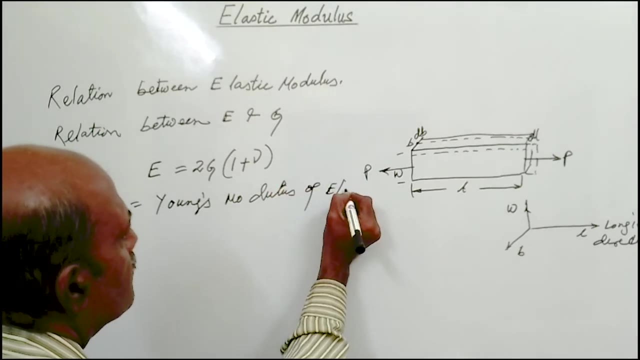 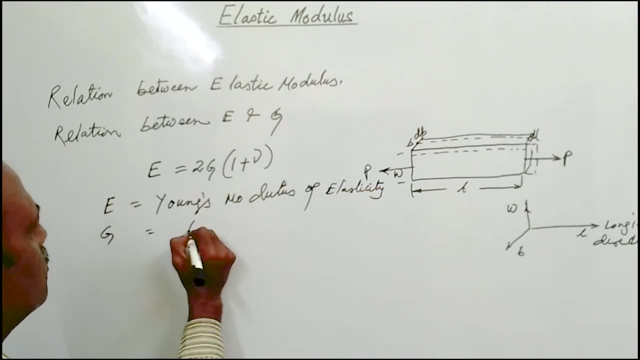 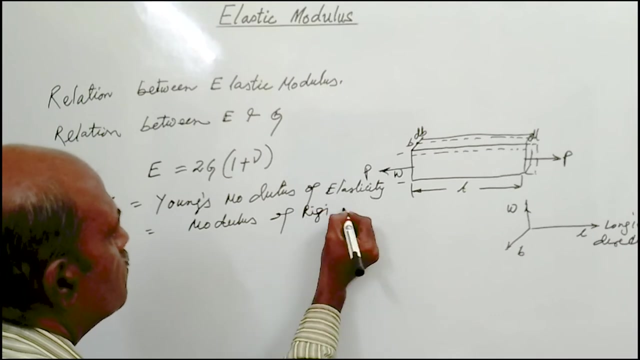 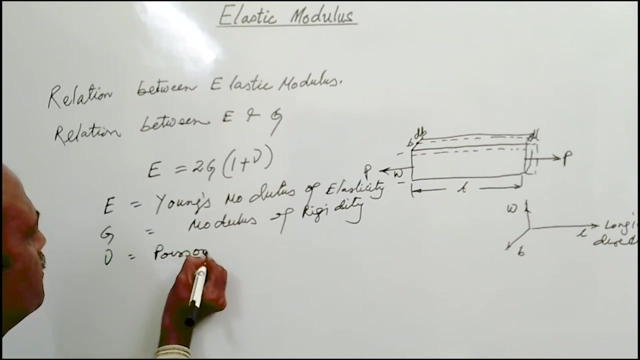 Young's modulus of elasticity and modulus of rigidity. that is, where E is equal to Young's modulus of elasticity, Modulus of elasticity G is equal to modulus of rigidity and nu is the Poisson's ratio. okay, so if any two is known, then the third one. 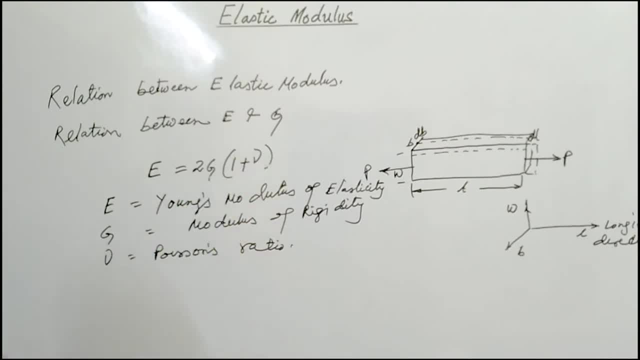 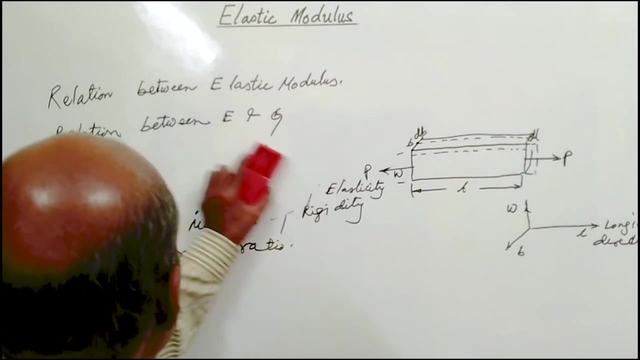 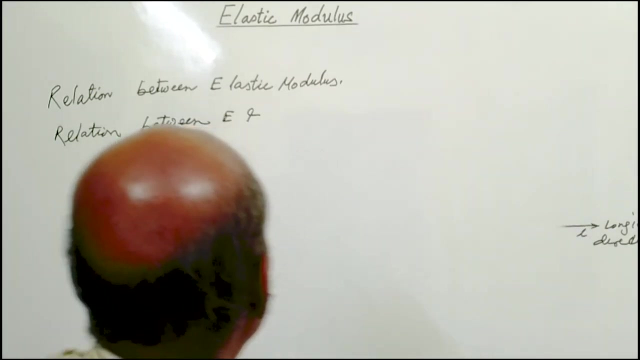 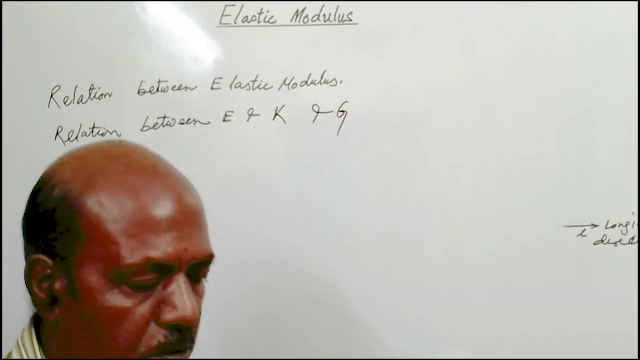 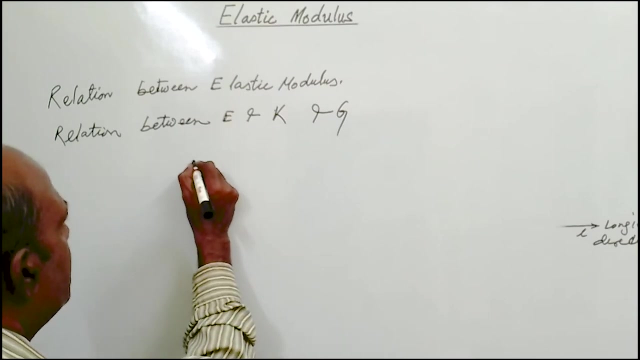 can be easily obtained. so that's why for isotropic material the properties can be completely defined if any two modulus is known. okay next. so you see the relation between EK and G, EK and G, E, K and G. So the relation between these three is given by. that is, E is equal to 9KG. 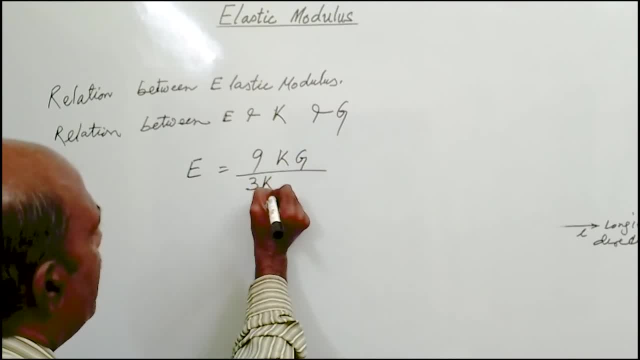 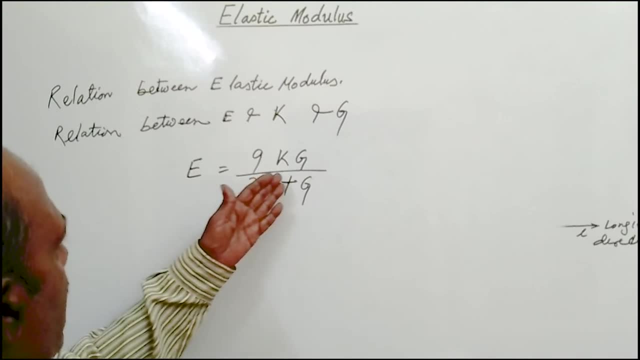 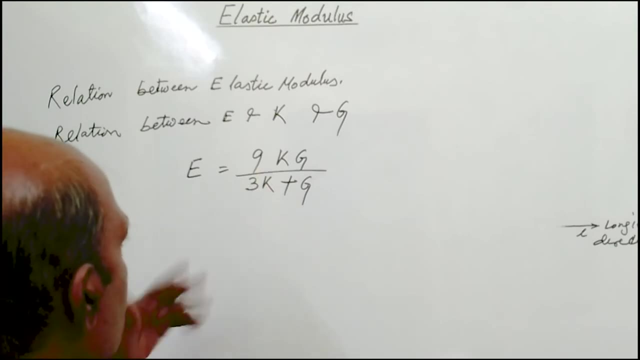 divided by 3K plus G. So this is the relation between E, K and G. So any two of these three are known. any two is known, then the third one can be easily obtained where E is equal to Young's. 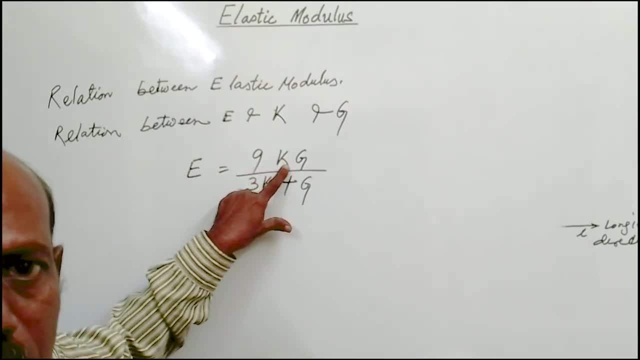 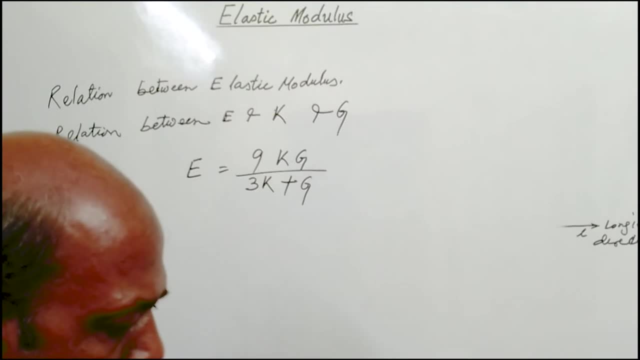 modulus of elasticity, K is equal to modulus of rigidity, bulk modulus of elasticity and G is equal to modulus of rigidity. And next, the relation, that is, relation between E and K. relation between E and K. the third one is: 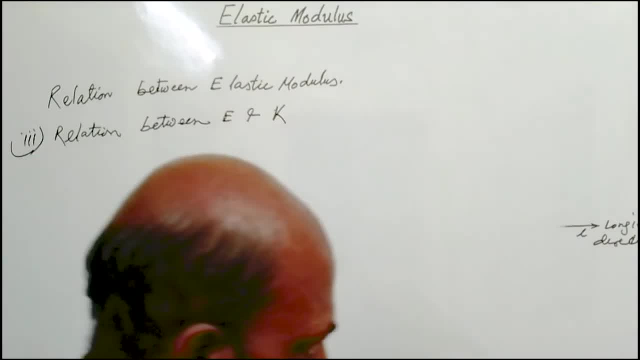 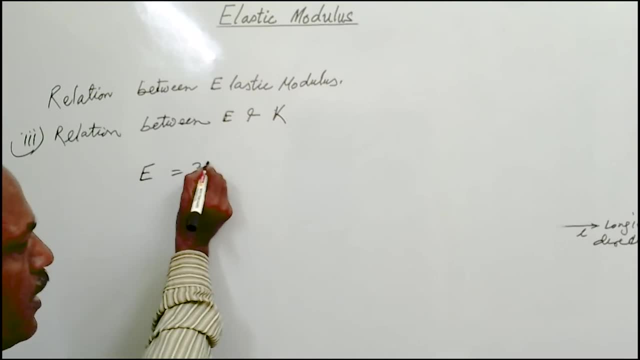 the relation between E and K can be written as: E is equal to 3K into 1 minus 2K. New, where E is the Young's modulus of elasticity, K is equal to the bulk modulus of elasticity and new is the Poisson's ratio. So these are the relation between the elastic constant and for isotropic material, two elastic constants are required to define the properties of the material completely. Now we will see The volumetric strain. the volumetric strain. so while defining bulk modulus, we have studied: 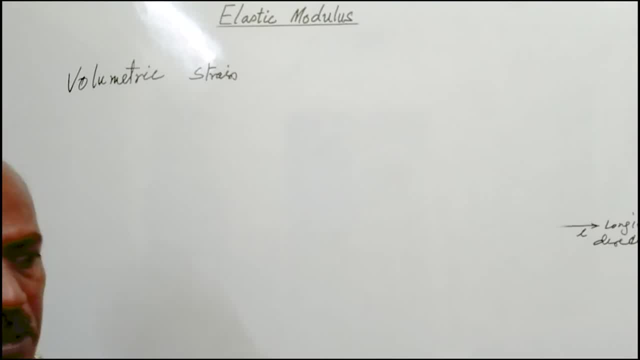 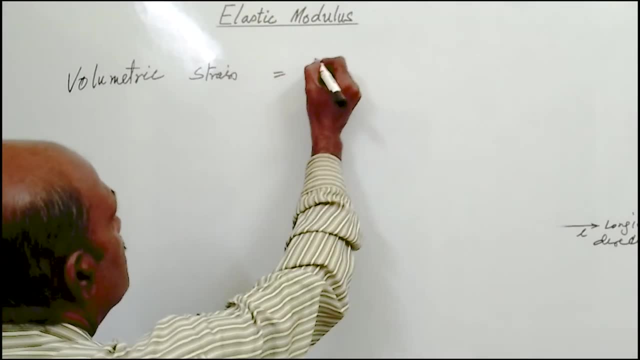 what is called the volumetric strain is equal to change in volume. volume, the volume, the volume, the volume of the volume is equal to the volume of the volume, Is it not? Yes, Yes, Yes, Yes, Yes. 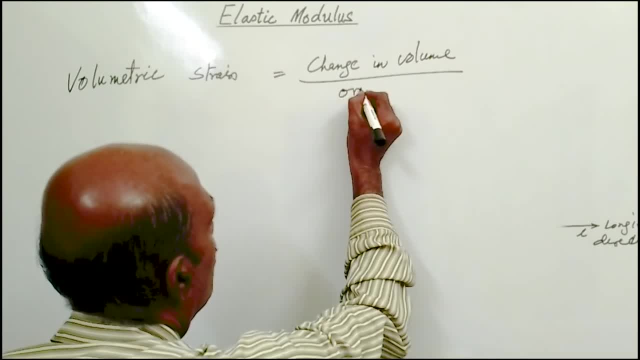 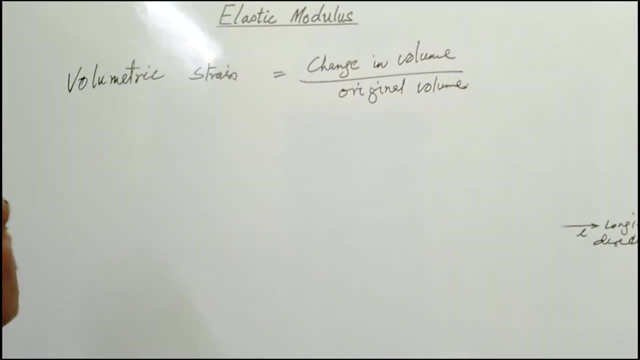 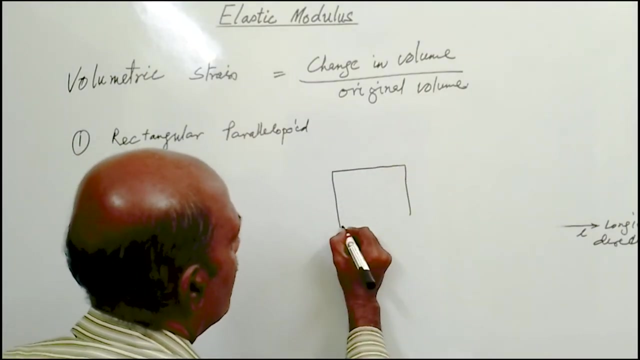 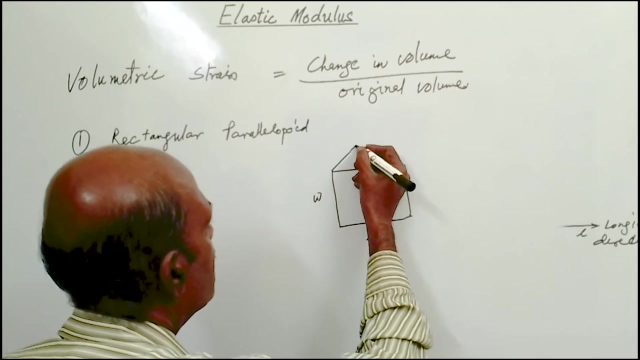 Yes to to original volume. now, how to find out this? so we'll see now. first one the case one: say a rectangular panel of white. so for this, say a body, rectangular body is given and the length of the body is l, width of the body is w. say thickness is w and width is b. 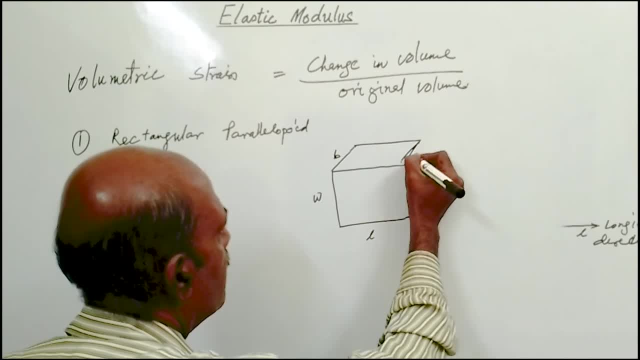 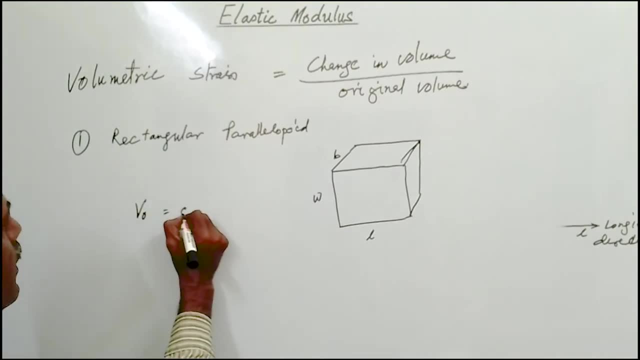 so for this, say, a body, rectangular body is given and the length of the body is l, so this is the body, this body is given. so original volume of the body, say v, o, is equal to original volume of the body and it is given by l, l into. 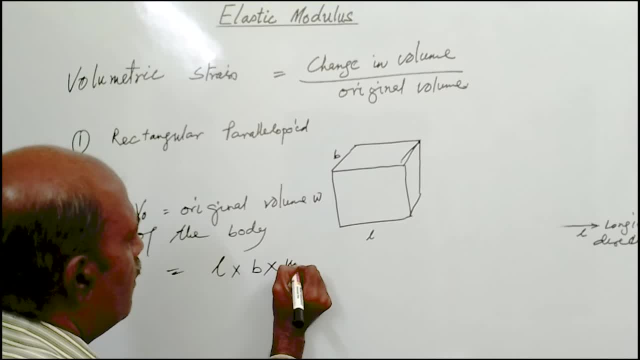 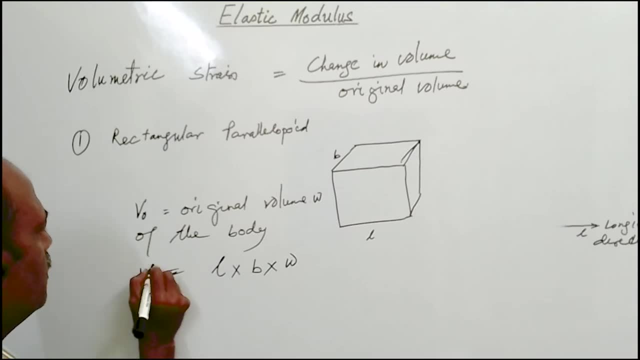 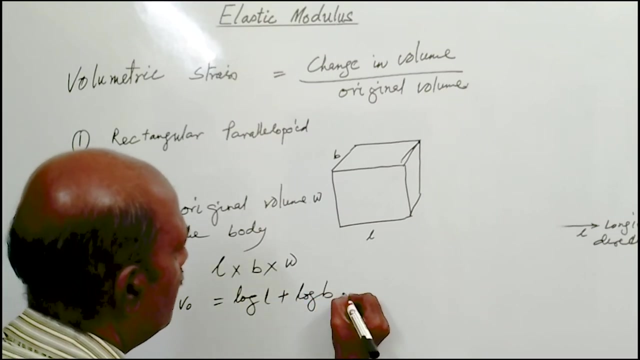 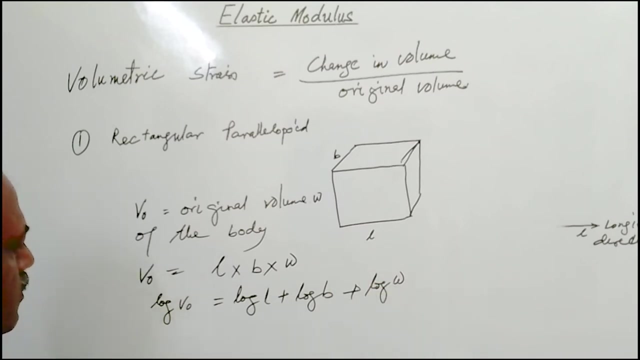 l into b, into w. so original volume of the body is given by l into b, into w. so this is your v o. so by taking log from both, the height, that is log v o is given by log l plus log b plus log w. now 'm writing this or taking the derivation so we can write. 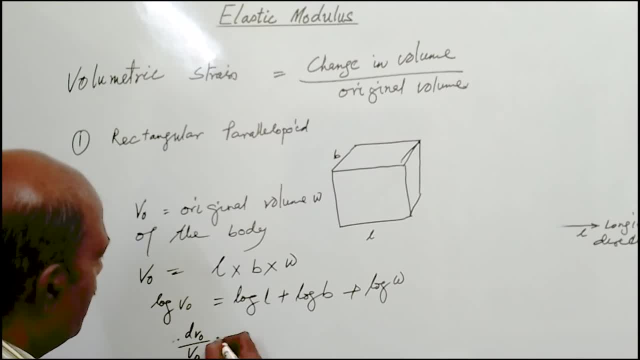 d v o by vo is equal to d l by l plus d v, by v plus d w by w. this is known as the volumetric strain changing volume. this is known as the volumetric strain changing volume. what will d be такую? ke focuses a volume. 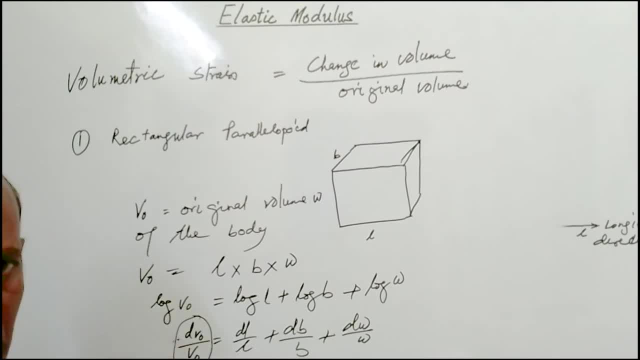 sigma. this is kenny. this is called volume. we say Ee over here b so we are going to to 소리 bosaurusarms price. another other accounts of you going to write see if you have any less. What is DVO? Because of the load acting over the body. change in volume is DVO over a volume of VO. So DVO to VO is the volumetric strain. 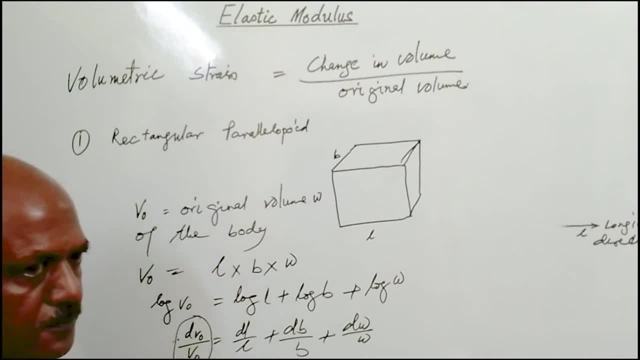 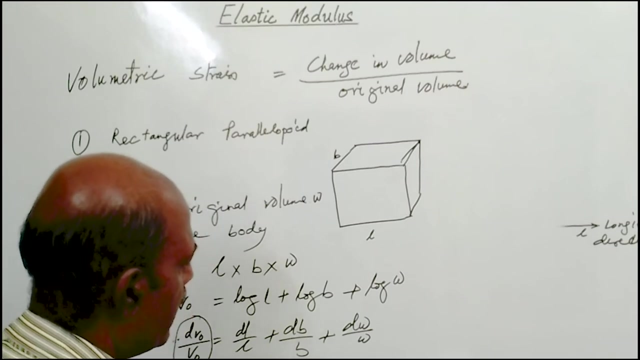 So we can write this one: as epsilon V is equal to DL by L, that is strain in L direction epsilon L, plus DB by B, that is strain in D direction, that is epsilon V, and DW by W, that is strain in W direction epsilon W. 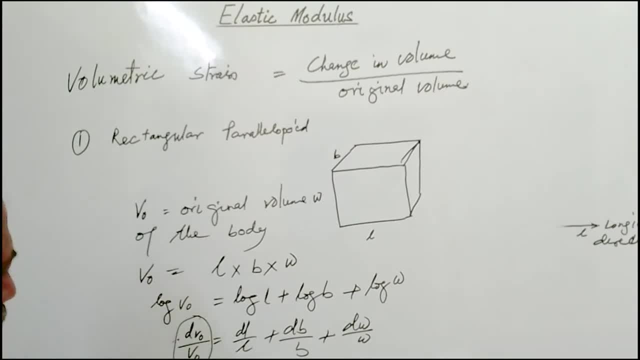 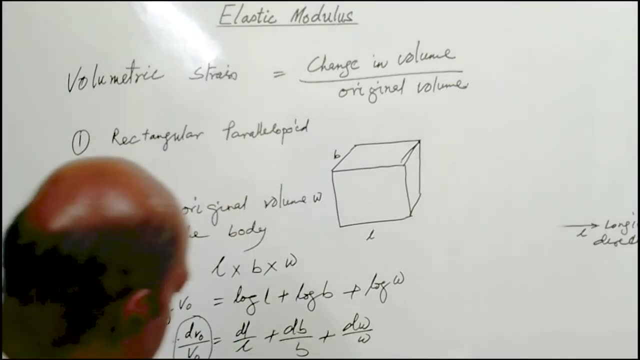 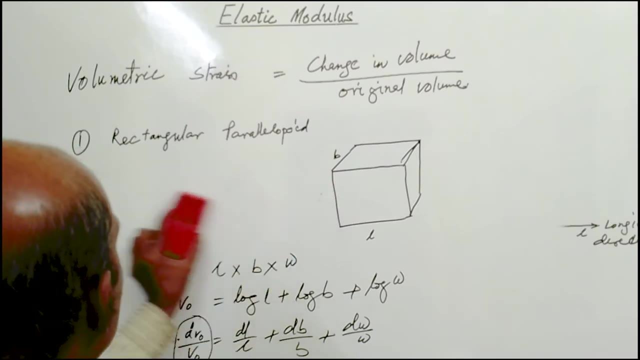 So epsilon V, that is, train in W direction. So this change in volume is given by epsilon L plus epsilon B plus epsilon W. that is the sum of the strains produced in L direction, B direction and W direction. Now we will see a cylindrical body. 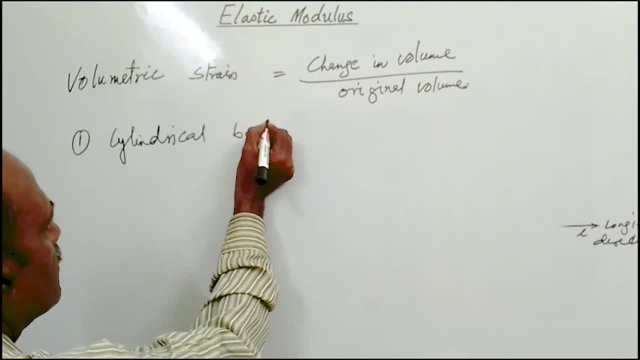 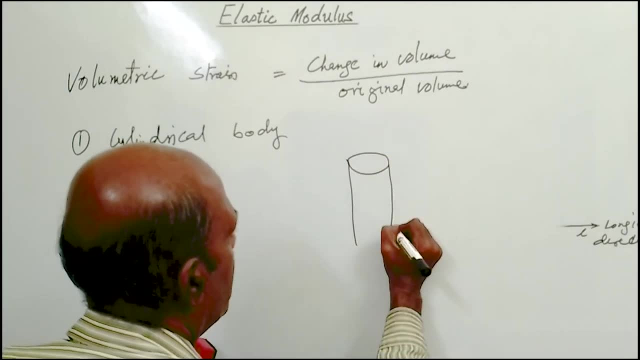 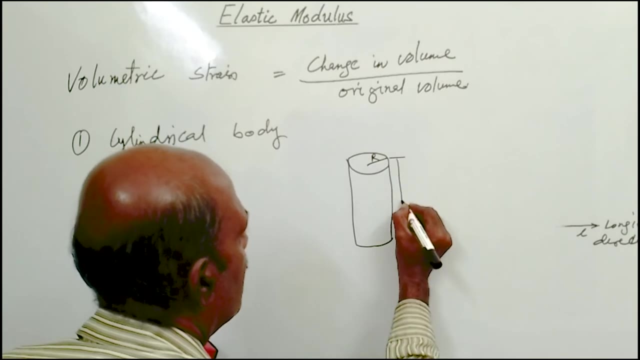 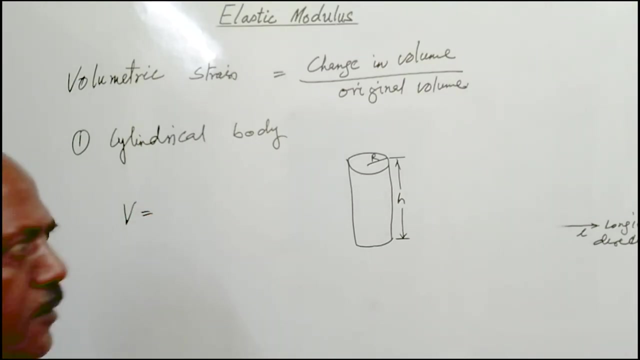 Say a cylindrical body of radius R, say radius is capital R and the height of the cylinder is. say H, H is the height of the cylinder. Now we can write: V is the original, The original volume of the body, that is original volume is given by pi. by pi R square into X. 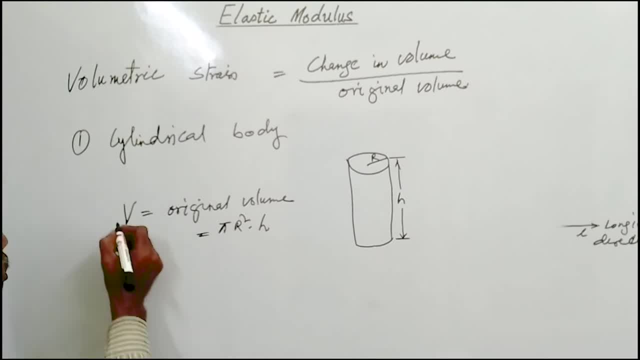 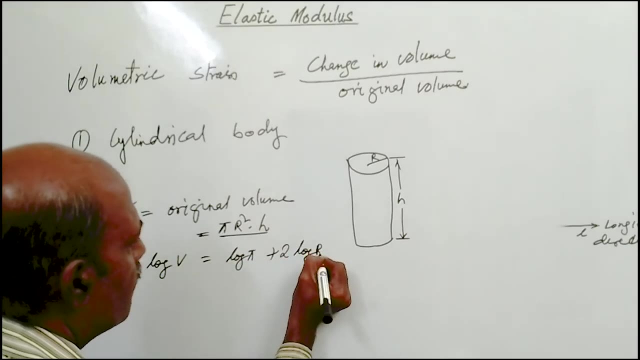 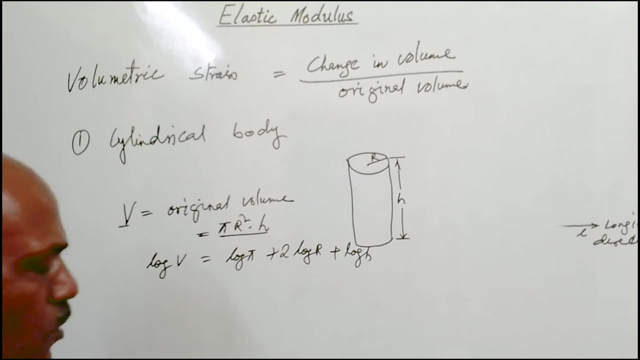 This is the volume of the body. So by taking log on both the side we can write: log V is equal to log pi plus Plus 2, log R plus log H. Now taking the derivation, so we can write or deriving this formula: 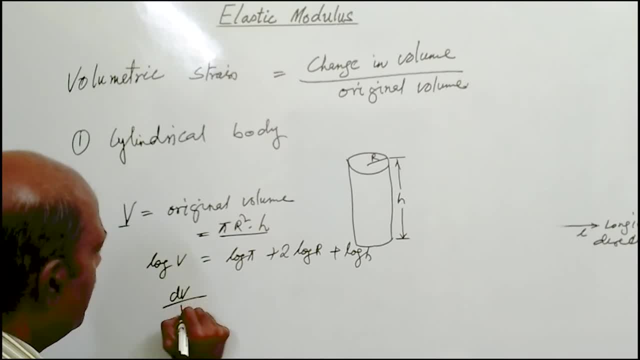 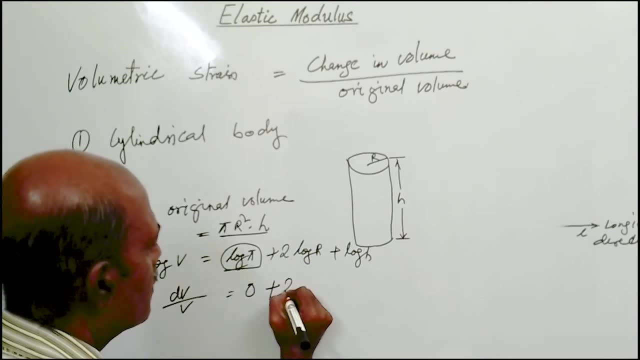 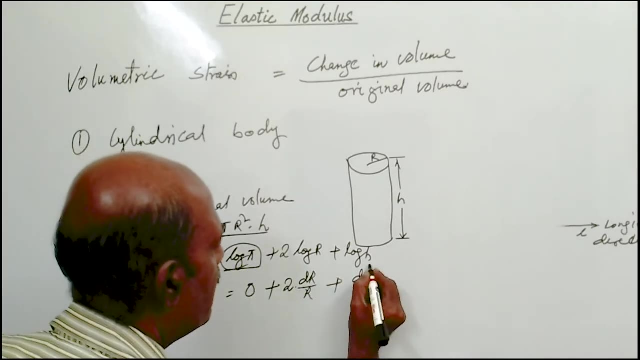 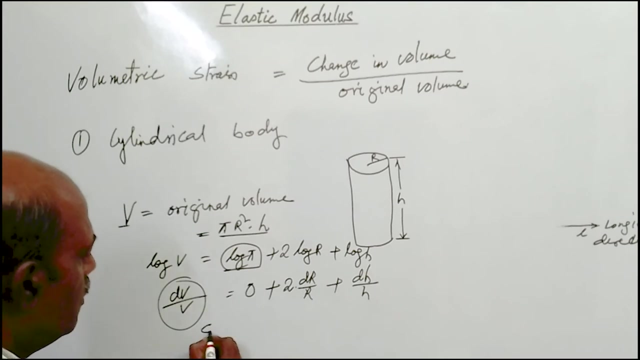 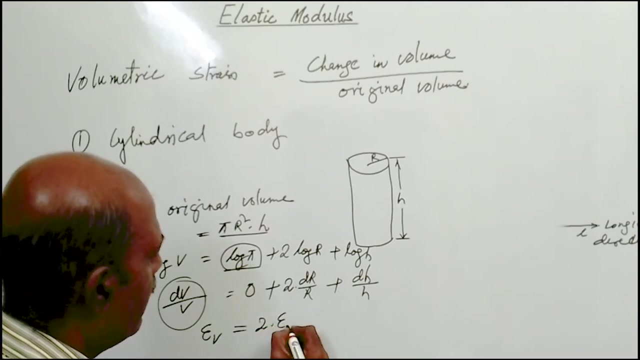 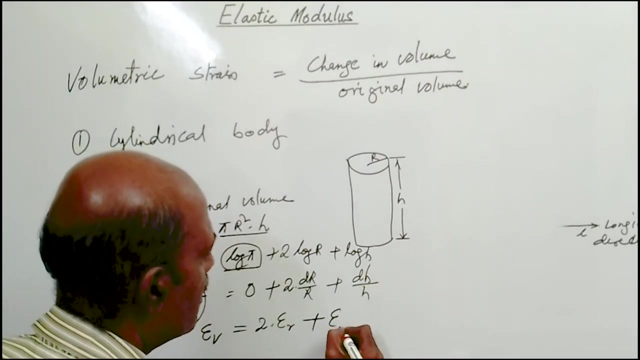 So we can write: DB by V is equal to derivation of a constant term. It will be 0 plus 2 DR by R plus DH by. So DB by V is known as volumetric strain is given by 2 into epsilon: R strain produced in R direction plus DH by H, that is, strain produced in H direction. 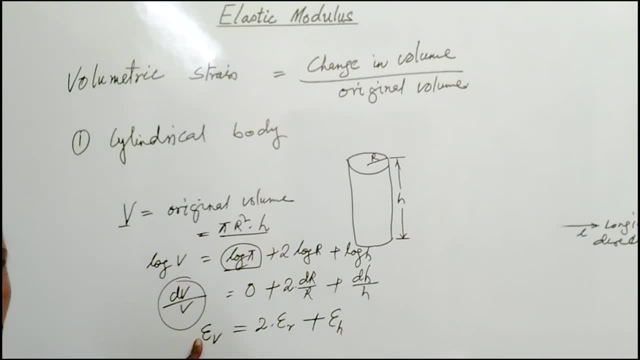 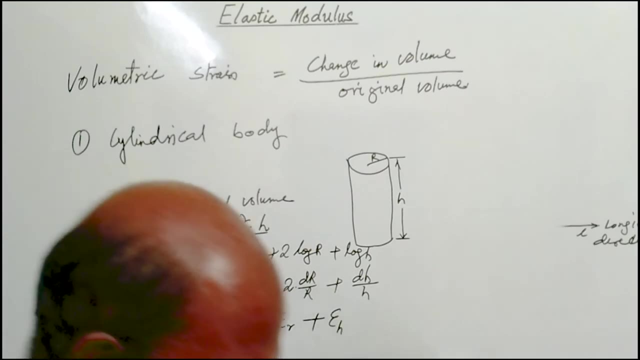 So epsilon V, that is volumetric strain produced in a cylindrical body, is given by. So epsilon V, that is volumetric strain, is given by 2, into epsilon R means strain produced in R direction, plus epsilon H, that is strain produced in H direction. Now we will see if the body is a spherical body. 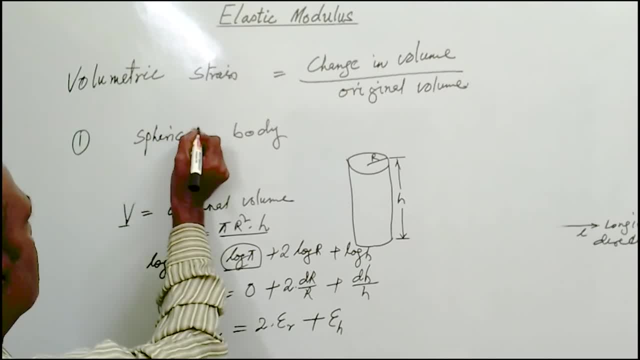 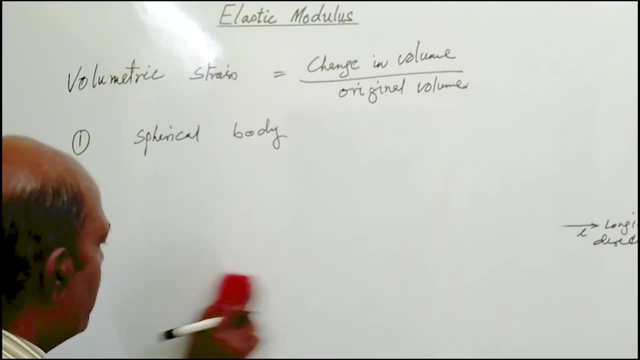 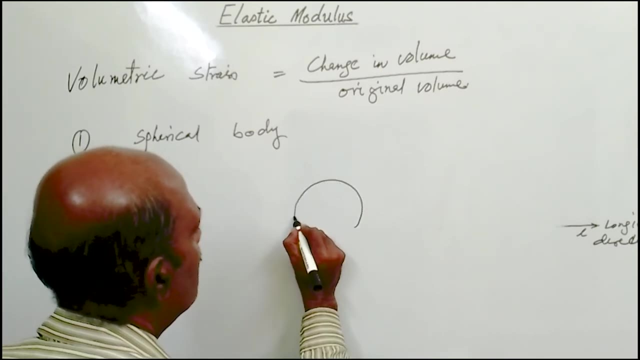 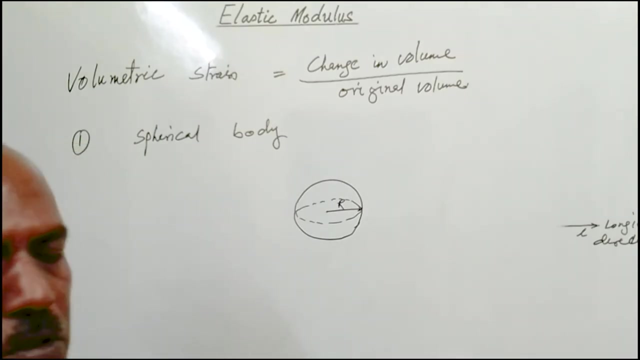 So if the body is a spherical body? So if the body is a spherical body, Let sphere of radius R. So this is a sphere of radius R And the sphere is under uniform stress intensity. Now, what is the volume of the body? 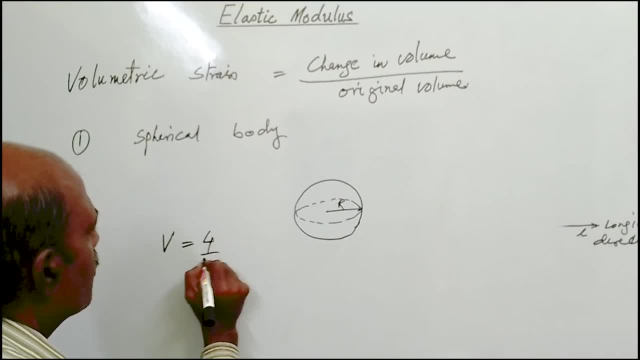 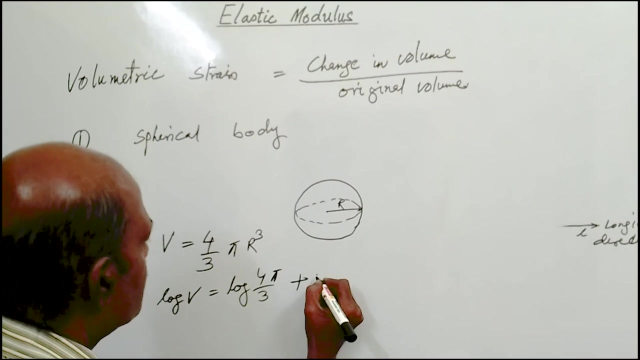 Volume of original volume is given by 4th R, by Into, say R, cube. So this is the volume of the body. Now, taking log on both the side, we can write: Log V is equal to log 4 by 3 pi plus log 3, log R. 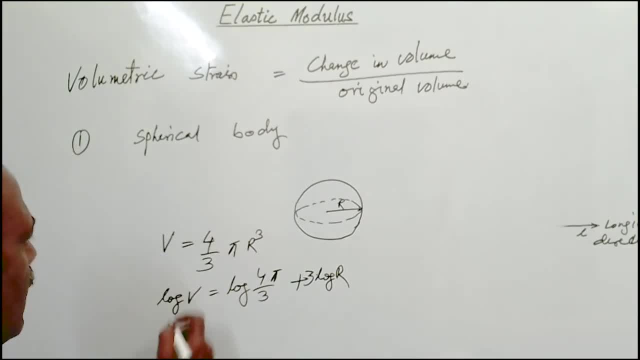 Now deriving this formula. Now deriving this formula We can write: dV by V is equal to: This is a constant term. So if you take log of this term, it will be 0 plus 3 into dr by R. Now what is that? dV by V? 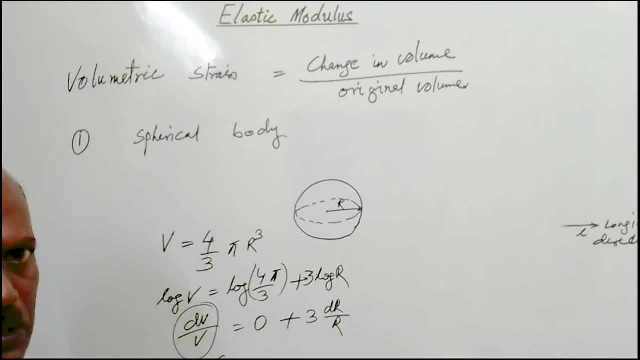 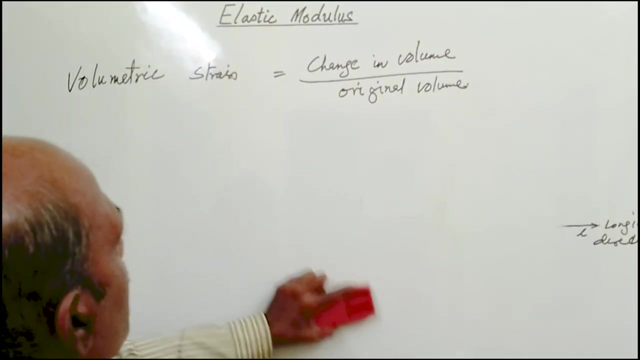 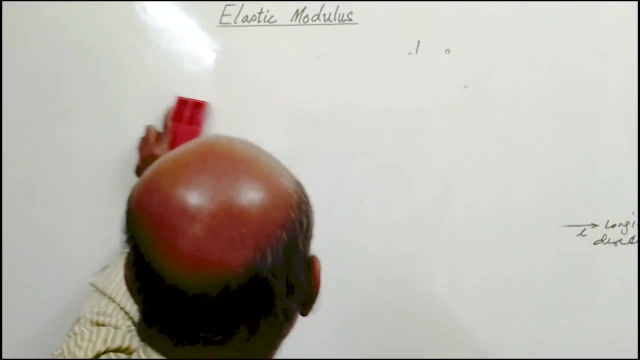 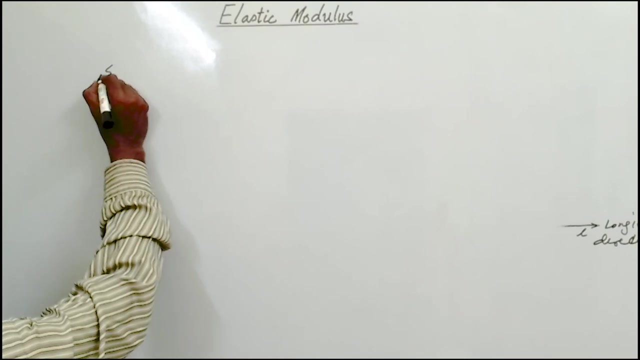 It is epsilon V that is volumetric strain produced in a spherical body Is given by 3 into R. given by 3 into epsilon r, that is radial strain. okay, now we'll see one more topic here that is not covered in the earlier videos. that is the stress and diagram. 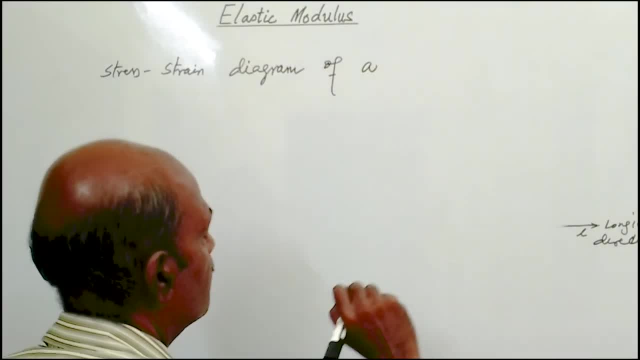 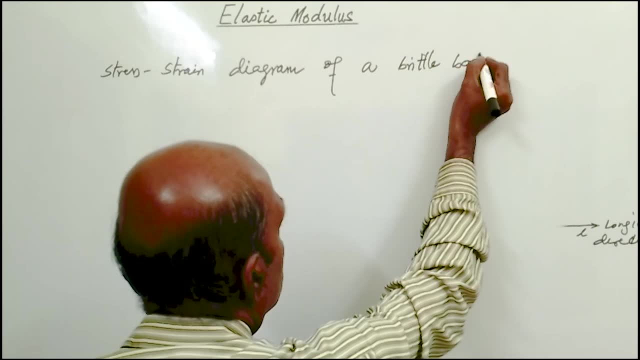 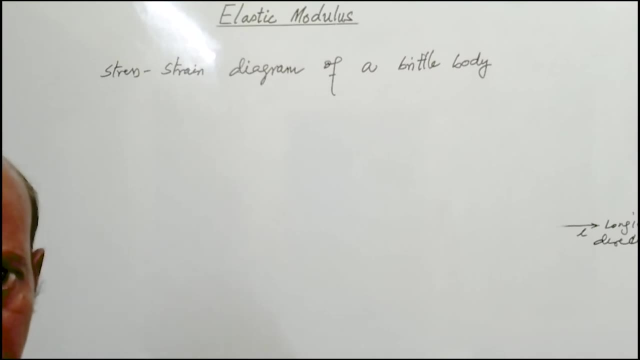 of a brittle body, so say a brittle body. so as far as the definition, what is a brittle body? the body which fails without much deformation, so that body is called a brittle body. so brittleness is the property, the body which is having brittleness cutting, that is called a brittle body, like cast iron, so without much deformation. the 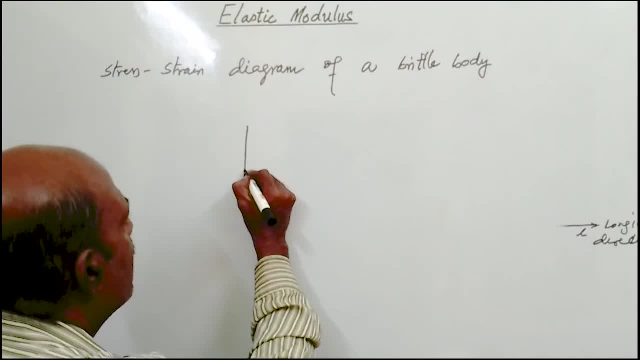 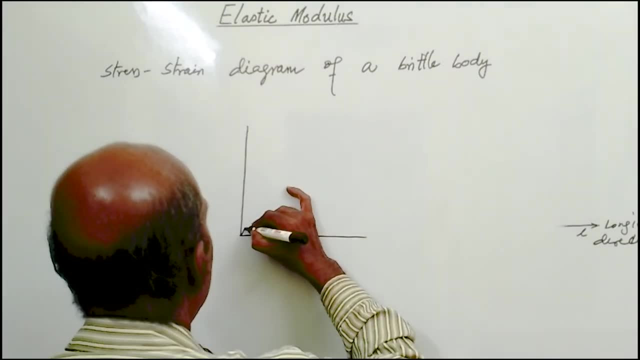 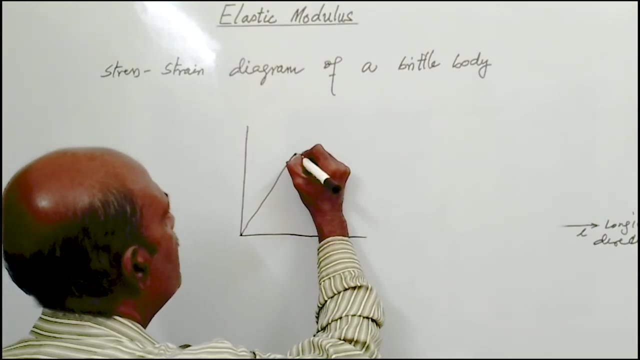 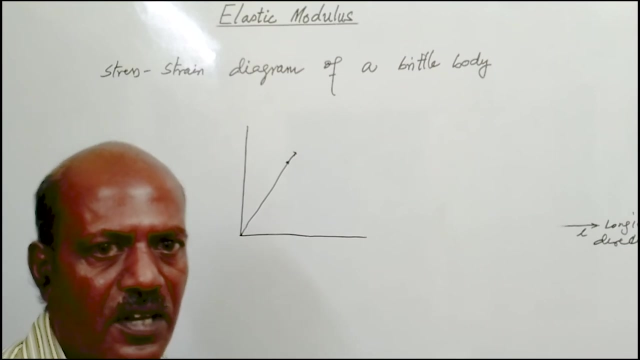 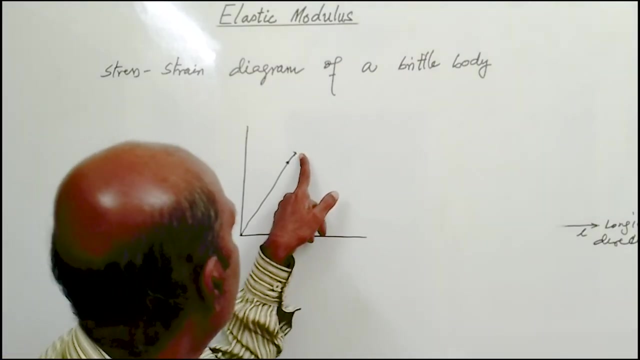 body fails. so if we see the stress and diagram of this body, say cast iron, if we see the curve will be straight line for some distance means up to proportionate limit it will be straight line. then it will slightly bend and fail. so not much information. stress-strain diagram: even the upper limit means Young's modulus, that is upper yield. 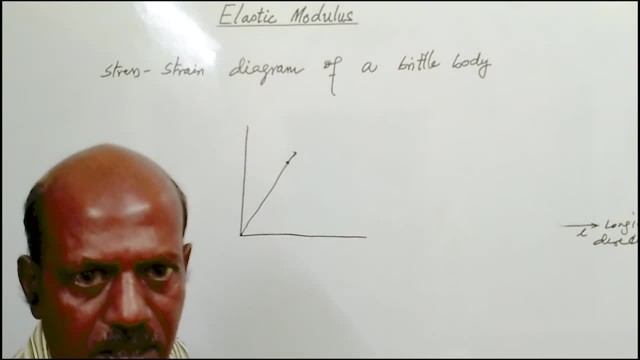 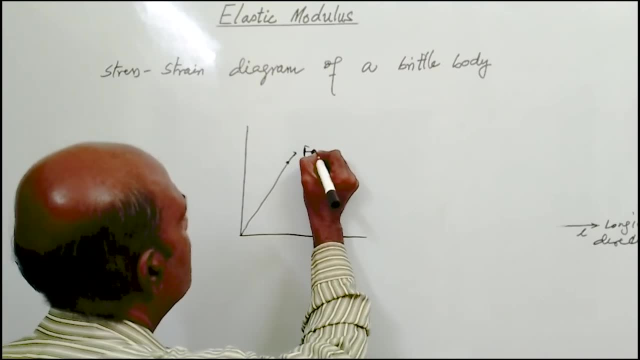 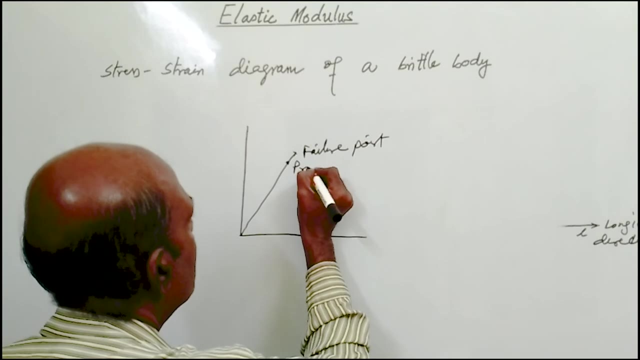 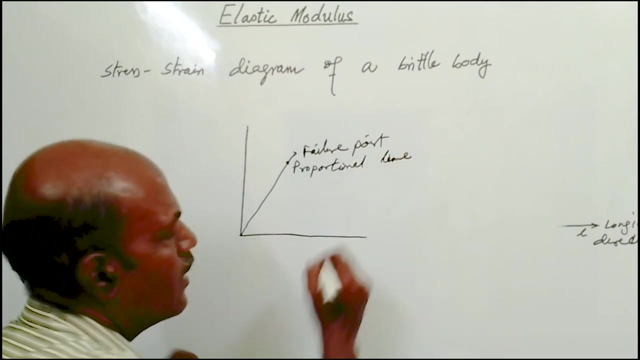 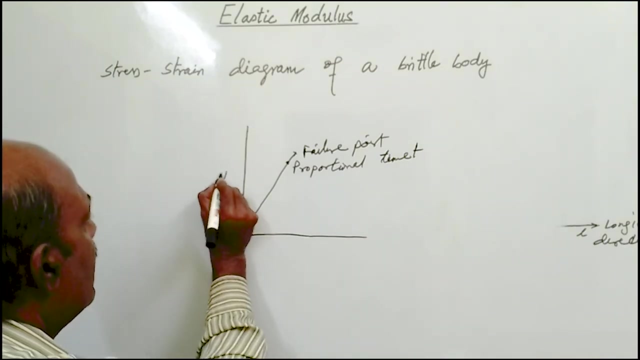 point is not clearly defined for this body, because without much deformation the body will fail. This is the failure point. Failure point, And this point is called the proportional limit. So up to proportional limit, the body, the curve is a straight line. 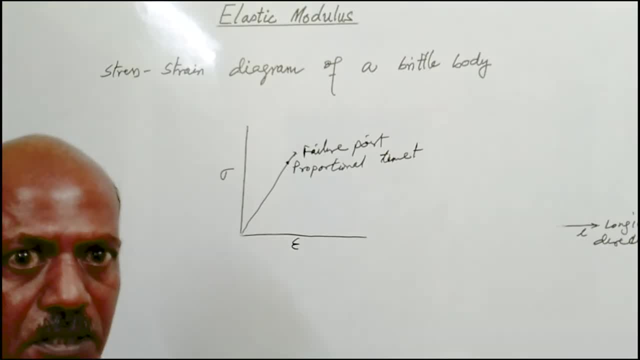 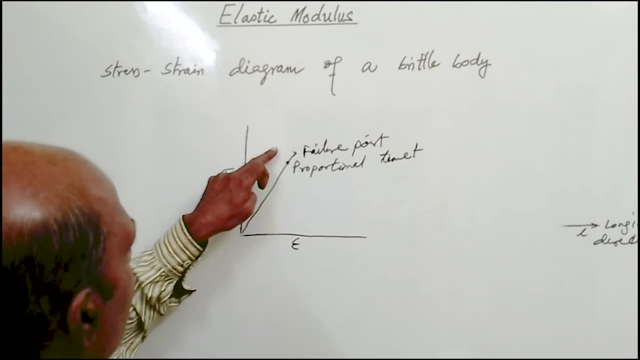 Up to proportional limit the curve is a straight line, And after that there will be very small deformation or no deformation at all and the body will fail. So even that upper yield point is not clearly defined. For this we are considering another term to to define yield point. 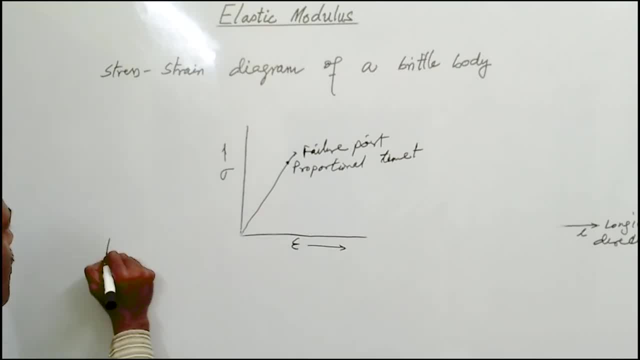 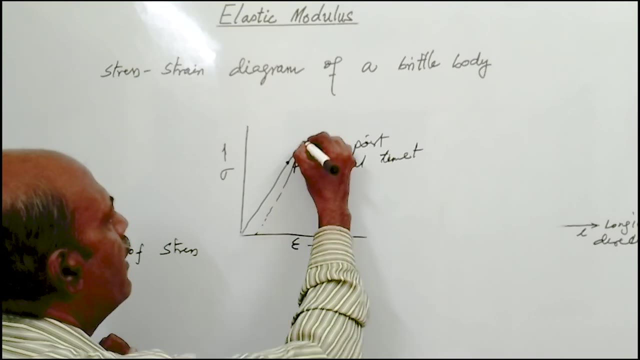 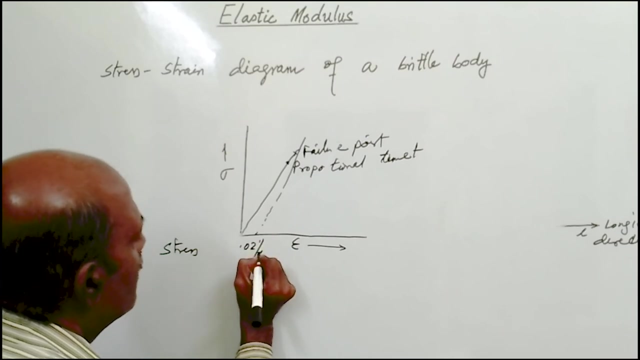 Okay, So that is called proof stress, Proof stress. So if we draw a line, So if we draw a parallel to this straight line, okay, that is, at 0.02% strain or deformation, 0.2% strain or deformation. 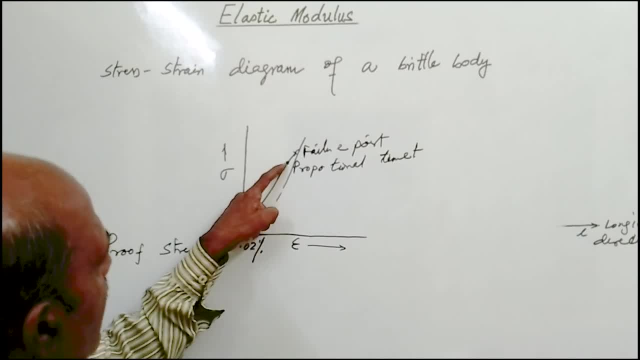 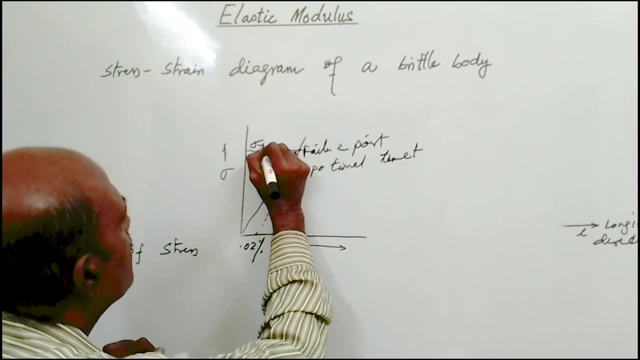 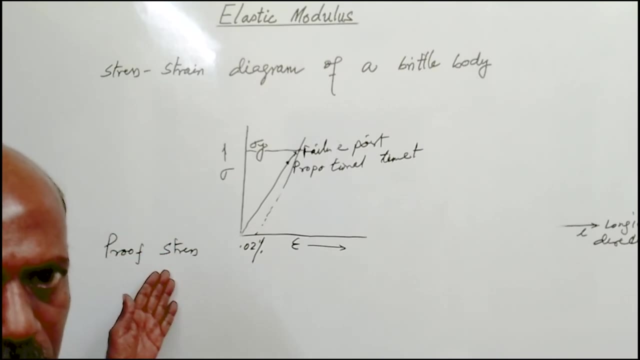 So if we draw a parallel line to this straight line, so this point will define the sigma y value of this. Okay, So proof stress is the stress value at 0.02% of the deformation. Okay, This is all about this topic and we will meet in the next video soon with some interesting 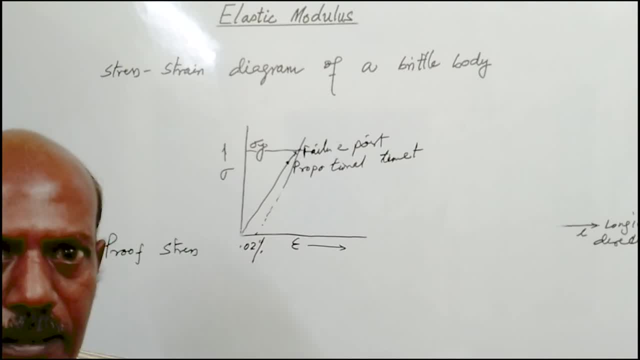 topic. So be connected with us: Like, share, subscribe and give your valuable feedback so that we could improve our video. Thank you, That's all for today's session. We would continue further on this topic in the next session. Keep being connected with us and ask any question in the comment section. 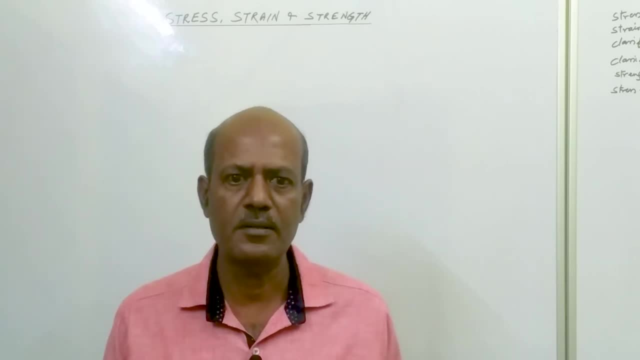